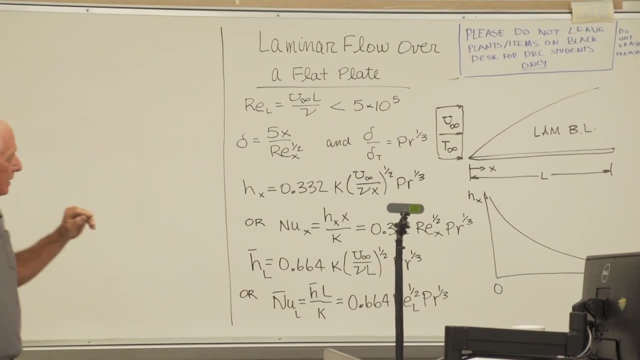 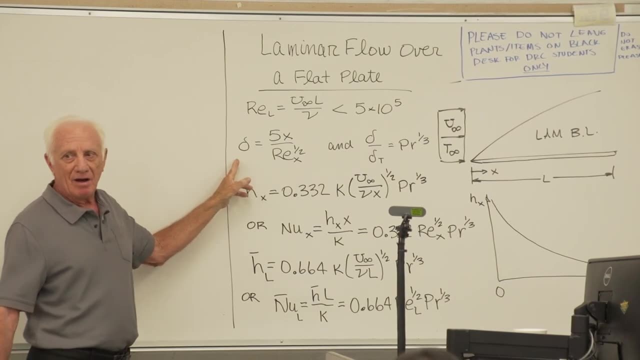 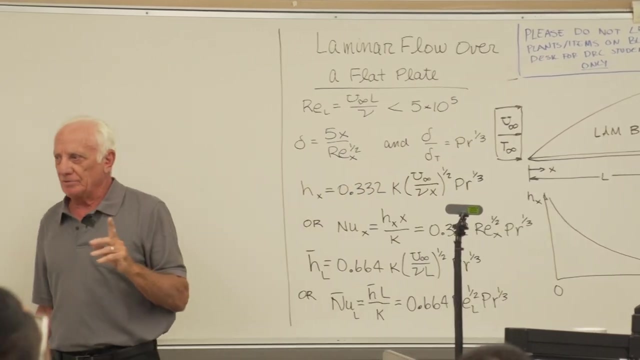 number is less than 500,000.. Two equations first, we did previously. First one gives us the velocity boundary layer thickness at any x value. The second one gives us the temperature or thermal boundary layer thickness at that x value. Ratio delta over delta. 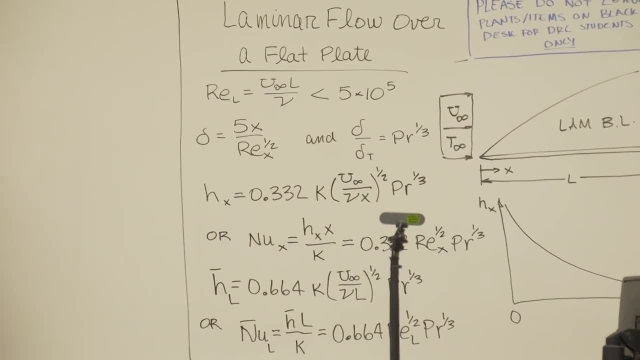 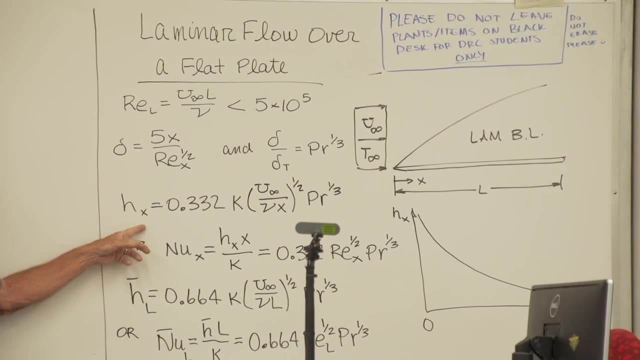 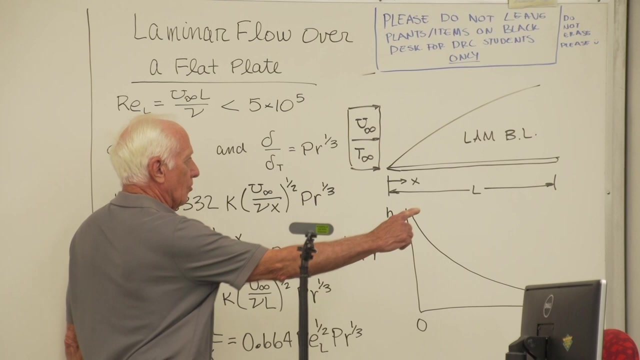 Delta t equal to the one third. Then we went through and we found the local convection coefficient. Local means x at a particular x value. So here's the plate over here, If it's a laminar boundary layer and someone says what's the local convection coefficient? where my 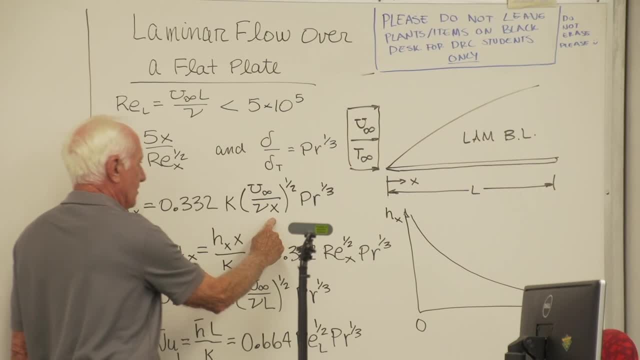 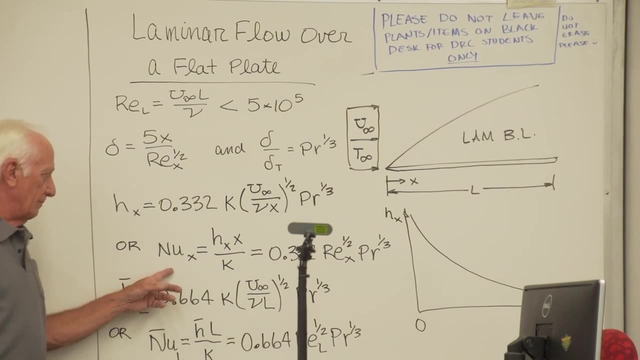 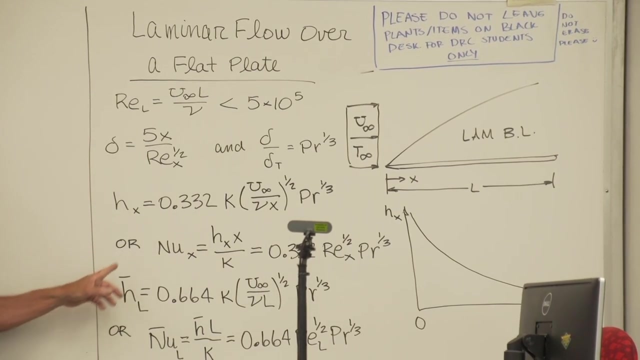 fingertip is: Put that x value in that equation and get h sub x. You can then define a Nusselt number subscript x, h sub x. This is called the local convection coefficient. This is the local Nusselt number multiplied by x divided by k of the fluid. If you want to get the average value of h, 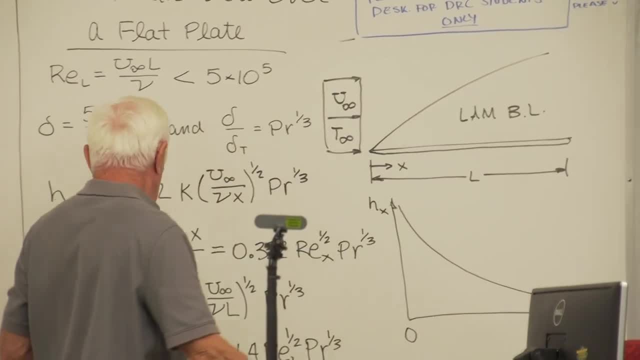 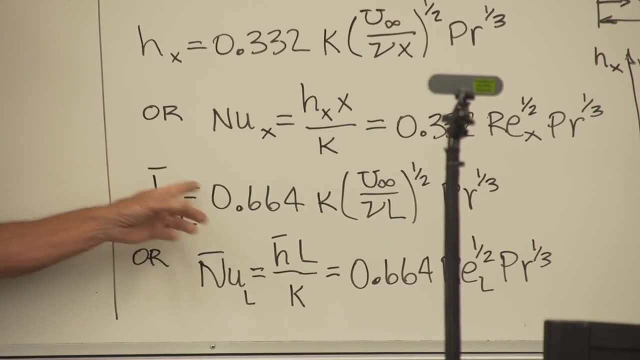 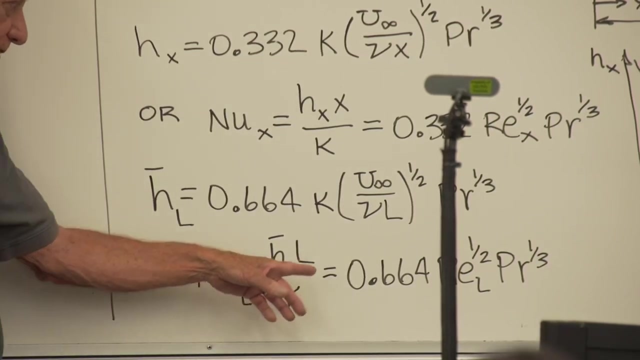 over the plate length l, then use this equation: h l bar. The bar means average. Average is this: And if you want to express it in dimensionless terms, then you've got the Nusselt equals 6, 6, 4, Reynolds to the one half, Prandtl to the one third, A dimensionless form of the equation. 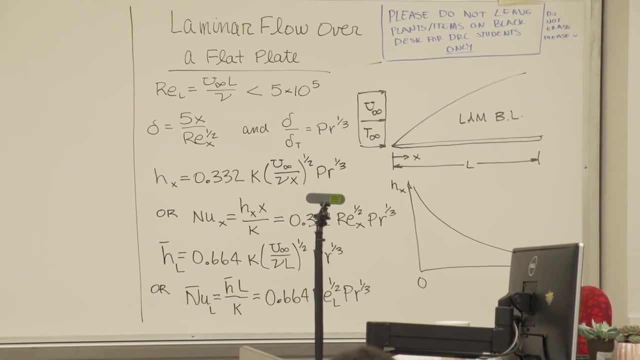 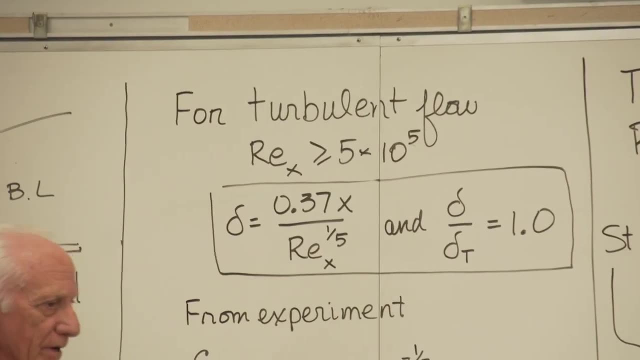 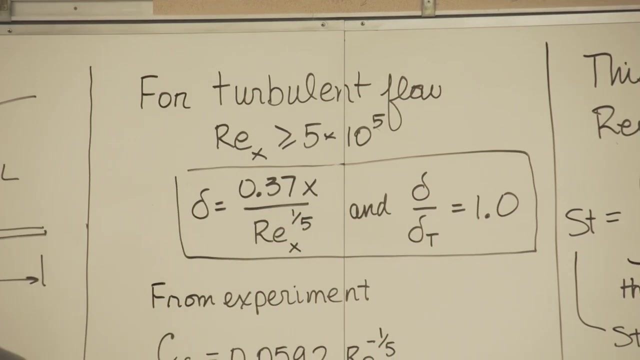 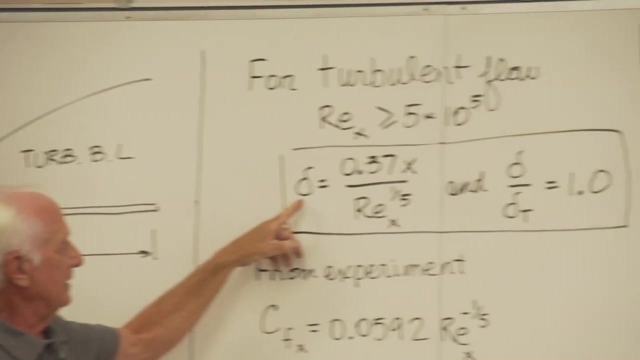 Okay, so that's where we left off last time. So, as we mentioned last time, now we're going to look at turbulent flow. So turbulent flow, the Reynolds number is greater than 500,000.. Here's the picture. Turbulent flow from x equals zero. If that's the case, this is the boundary layer: thickness, delta. 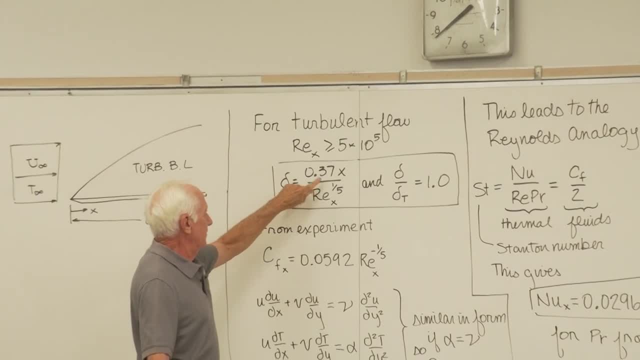 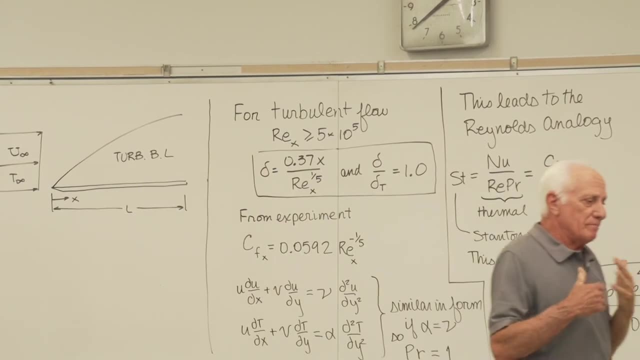 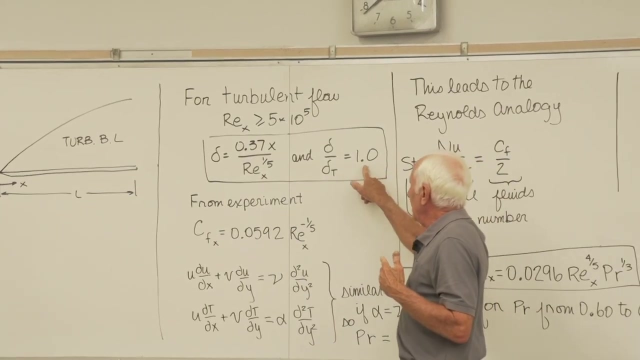 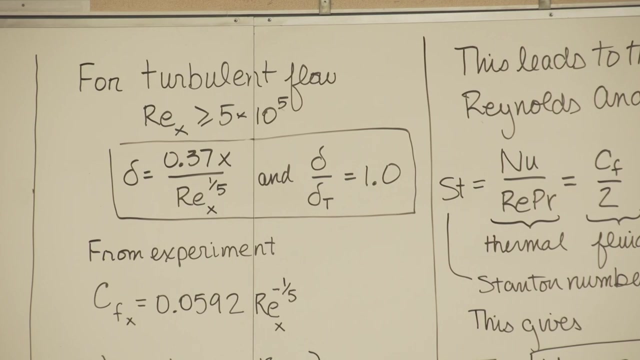 Very similar to laminar flow. The constant is different and the power of x is different. But turbulent flow, there's a lot of mixing that occurs. So it turns out that delta over delta t is one for turbulent flow. Well, the velocity boundary layer thickness is about equal to the temperature or thermal boundary. 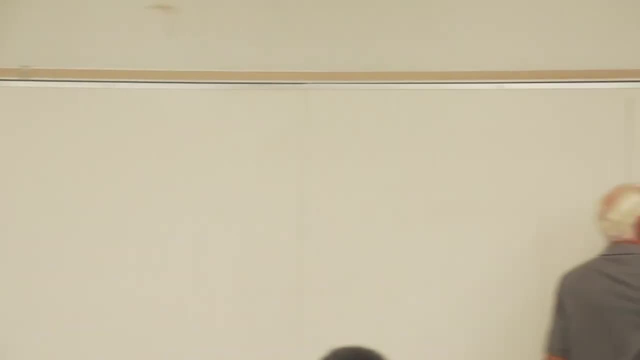 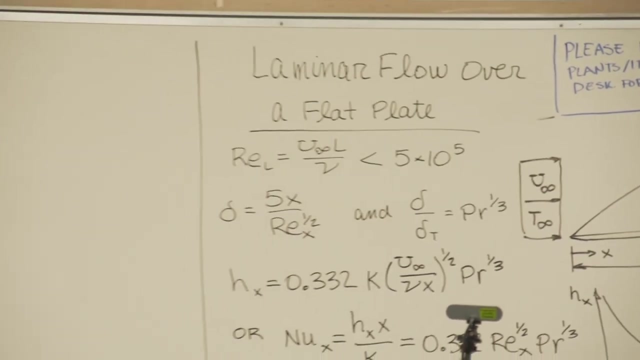 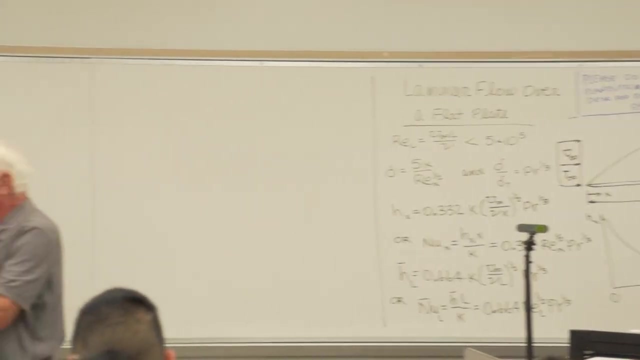 layer thickness. Laminar flow: that ratio was Prandtl to the one third. We solved the laminar flow equations Pretty much. It was done mathematically. When you get to turbulent flow it's very complex, very difficult. It's not done mathematically. 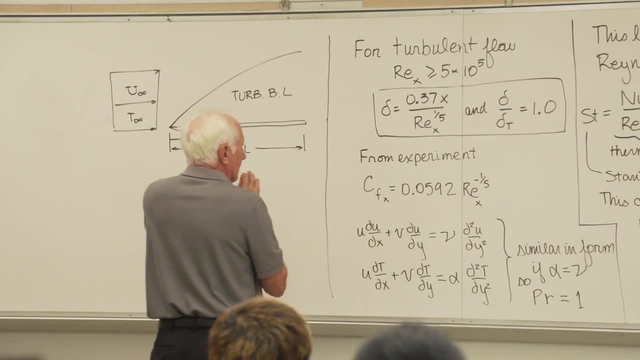 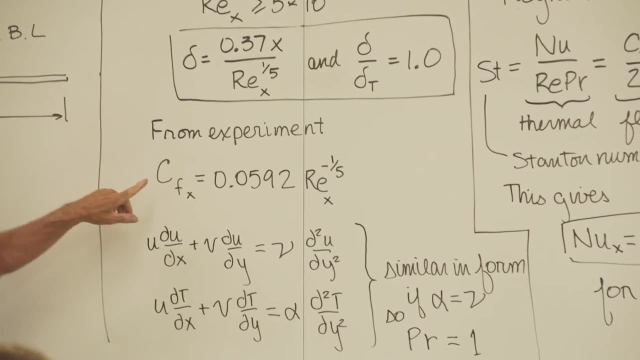 So we have to do one more thing here. We have to do the fundamental of the equation, which happens to be the. we have to walk our way through it. You start off and from experiment. this is done experimentally. They found out this to be true. 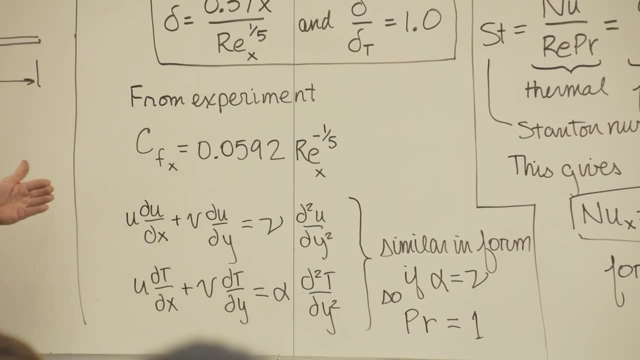 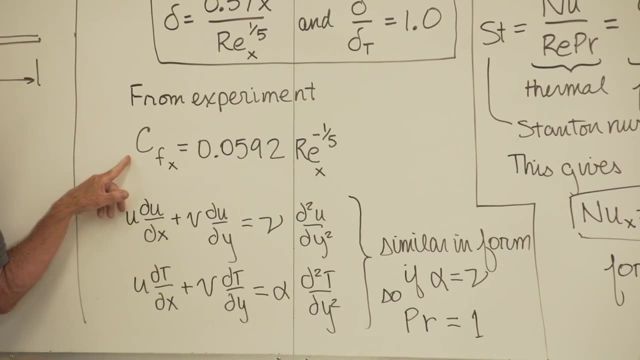 Now Cfx, go back to your fluid mechanics. This is the. x means local, f means friction, c means coefficient. This is the local skin friction coefficient: dimensionless: 0.0592 Reynolds to the minus 1.5, experimental. 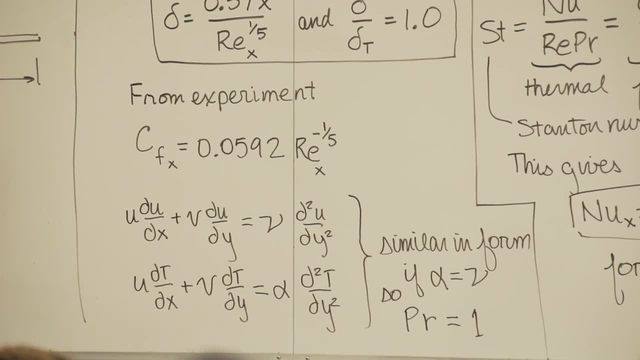 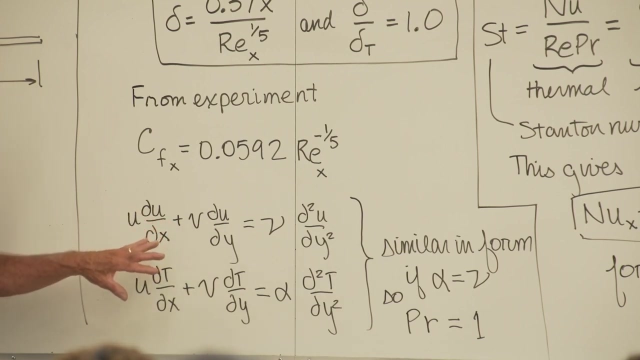 Then they said: you know what? We had these two equations on the board a couple of class means ago. The one is fluid mechanics, the other one is the thermal equation with temperature. These two equations are very similar, except the one in velocity. 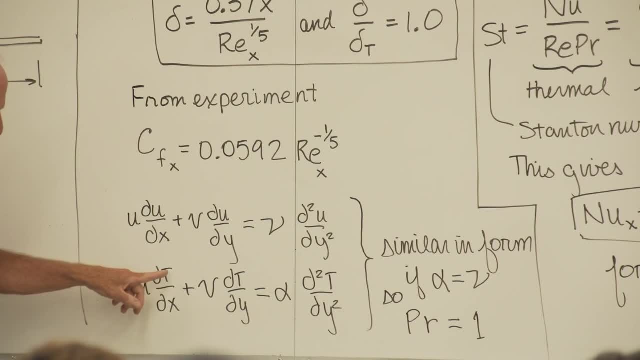 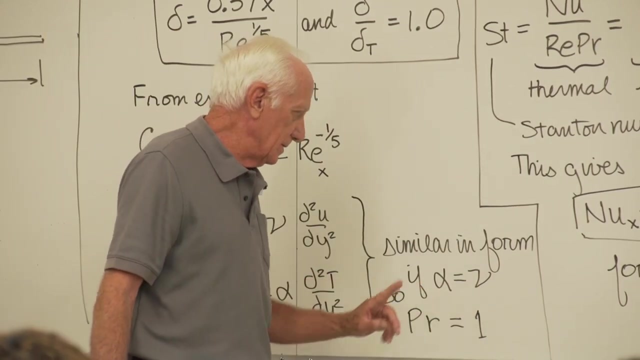 has u, u, u, temperature, t, t, t. They're very similar, just replace the u by a t. and especially similar if alpha equal nu. thermal diffusivity, kinematic viscosity: If that's true, the Prandtl number is equal to one. 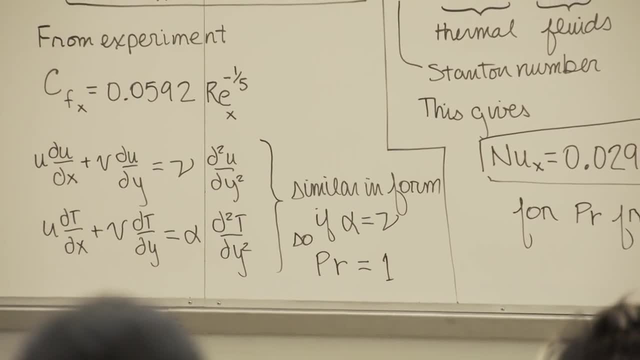 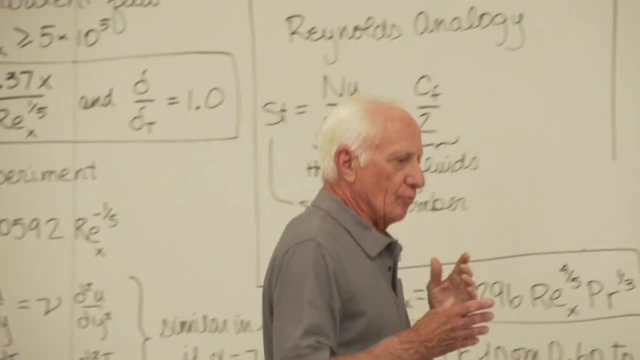 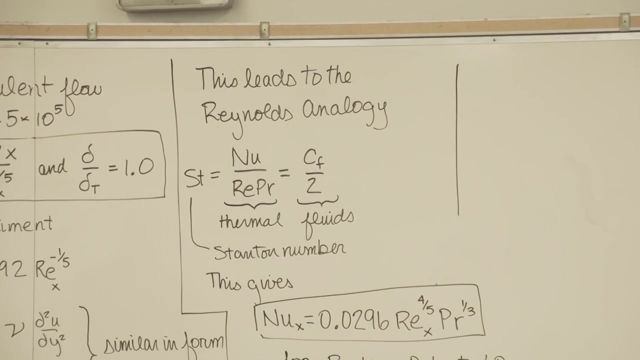 since the Prandtl number is a ratio of those two, These two equations look extremely similar. for Prandtl number equal to one, That leads to something called the Reynolds analogy. The textbook walks you through it in about a page. We're not going to spend the time for that page. 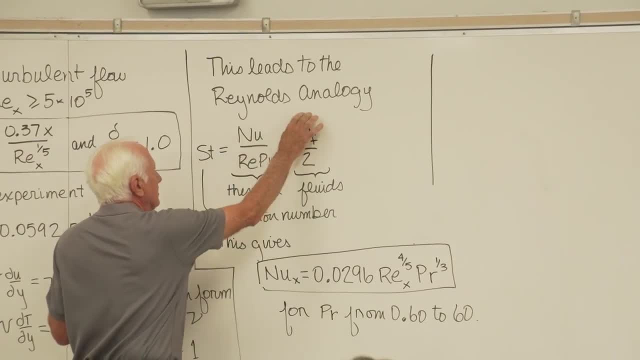 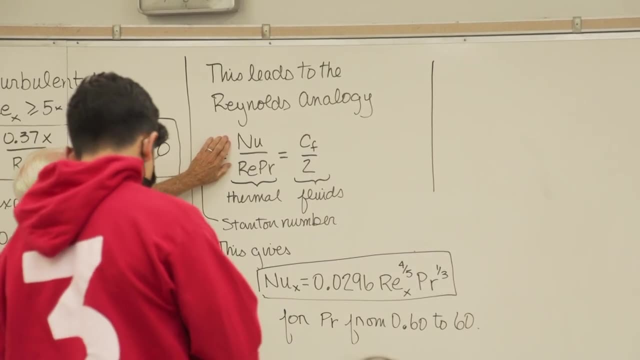 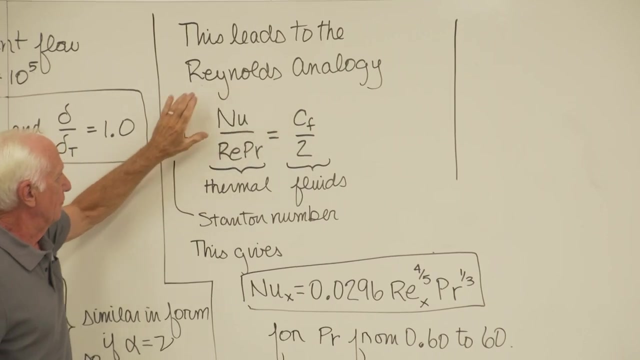 We're going to the result. The Reynolds analogy result is: forget that guy. now, Nusselt over Reynolds Prandtl equals CF over two. This gives us the Nusselt number in terms of the friction coefficient. Where does that friction coefficient come from? 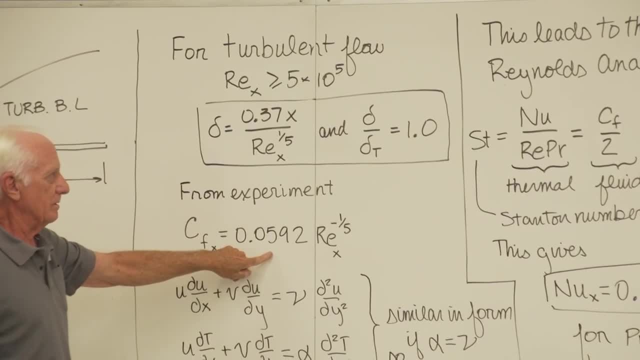 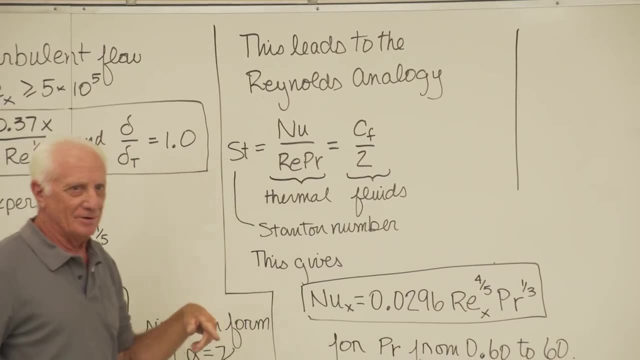 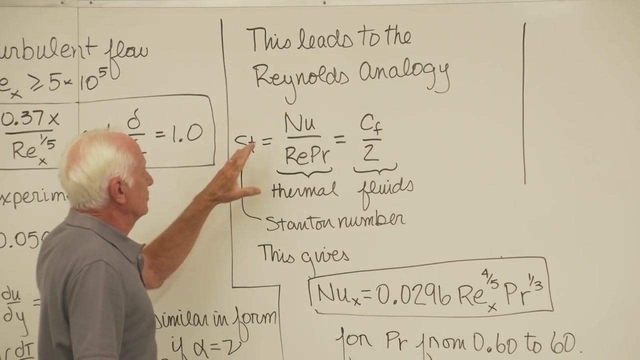 Experiment. here They define a new dimensionless parameter. It's called the Stanton number. as I told you, There's a ton of dimensionless parameters in fluids and heat transfer Stanton number. So this is called the Reynolds analogy. Take the results and experiment for friction. 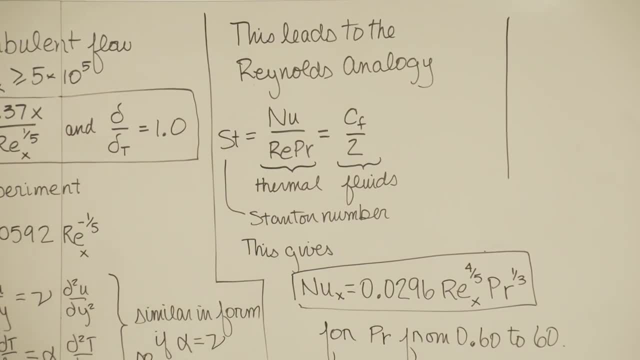 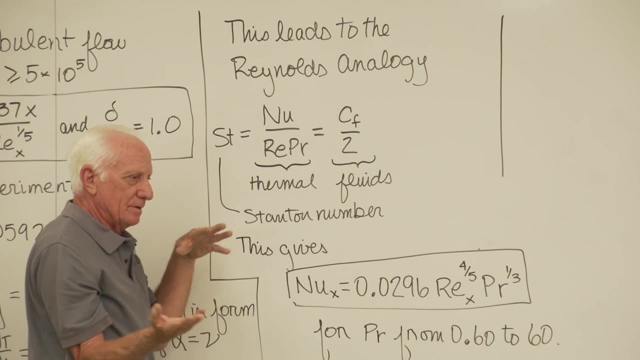 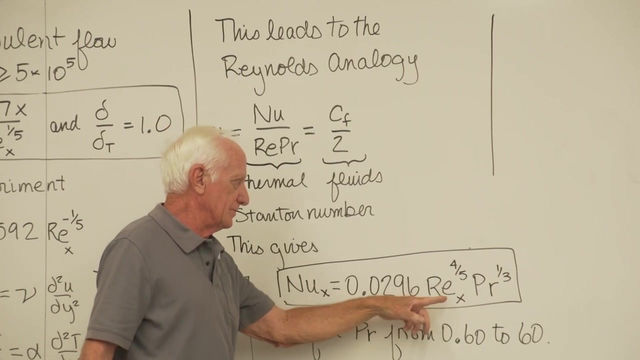 and equate that to something to do with convection heat transfer: h, H. If you go through that on that page I mentioned, you end up with the Nusselt number is this: 0.0296 Reynolds to the four-fifth, Prandtl to the one-third. 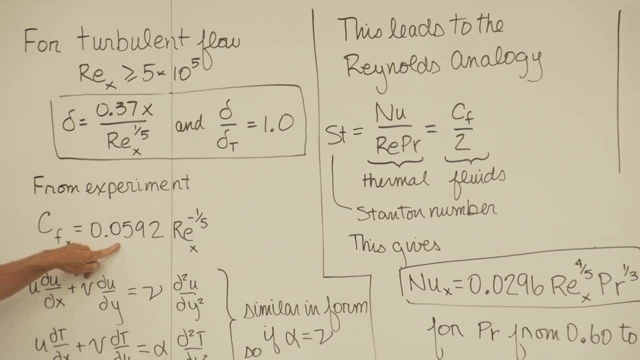 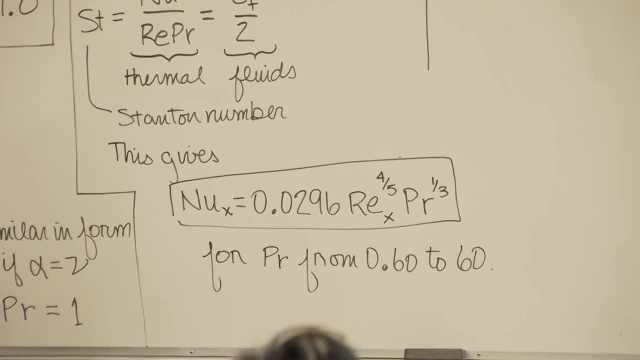 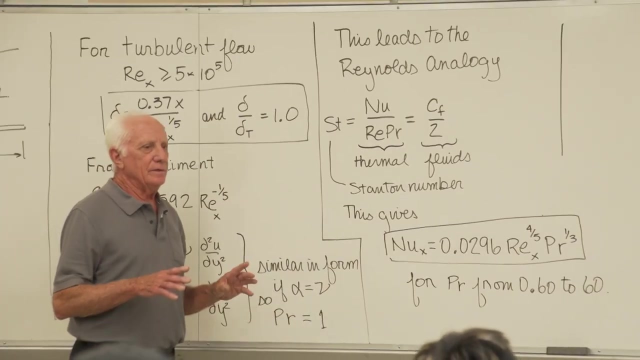 CF over two, what's 0.0592 divided by two, 0.0296,. so you could walk your way through it that way. Where did this Prandtl number come from? Because we said it's one? Well, yeah, 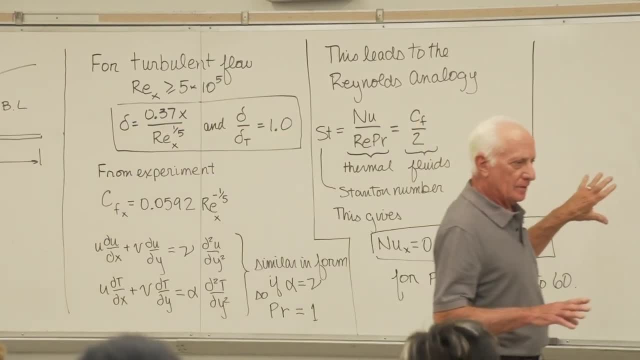 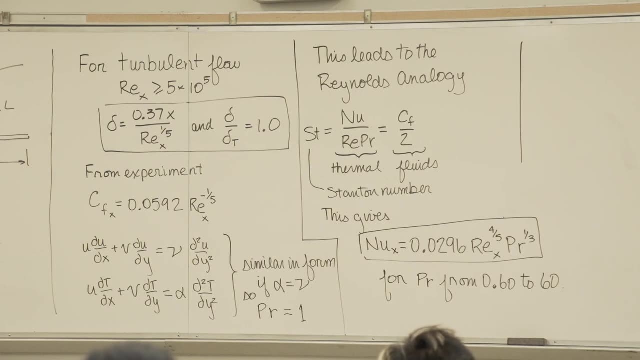 Reynolds analogy works out really good for Prandtl number equal to one. What's a Prandtl number for 300K? for air 0.7,, for water 6 point something. So most fluids maybe don't have a Prandtl equal one. 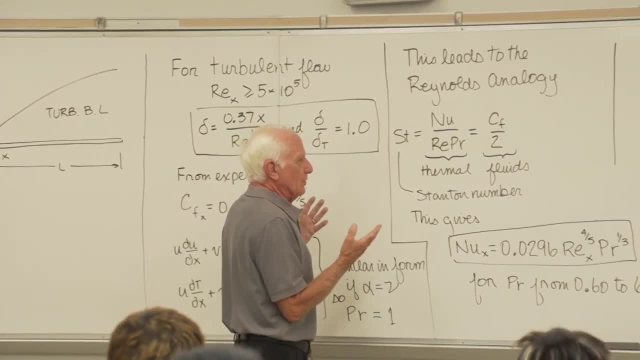 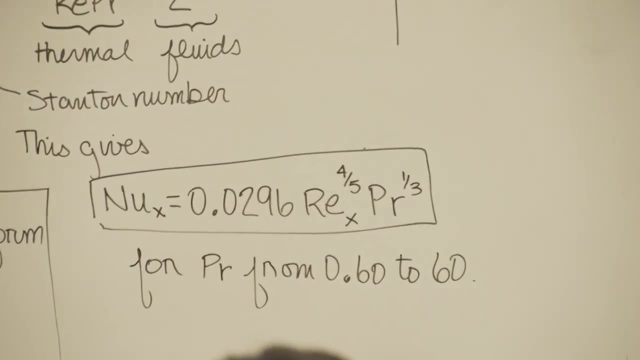 So what do we do then? if the Prandtl's not equal to one, The author says we throw in a correction factor. So we put this guy on the end of it to correct for property variations. Prandtl to the one-third. 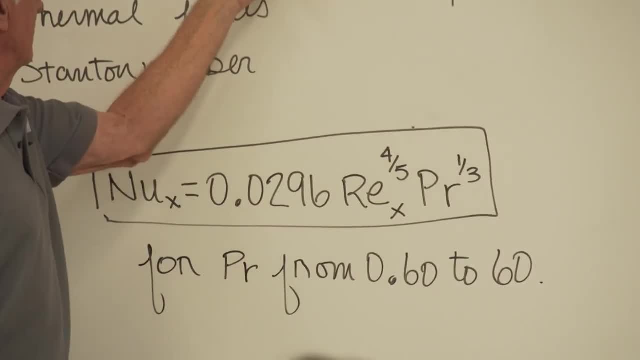 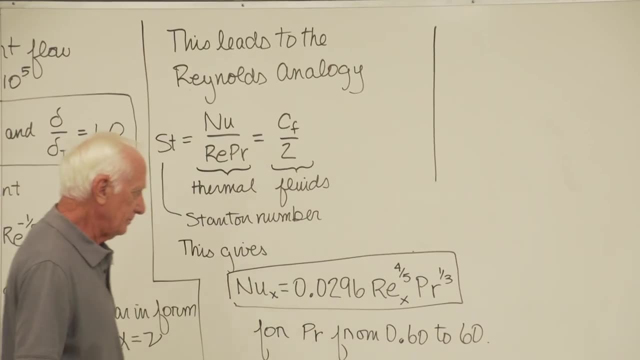 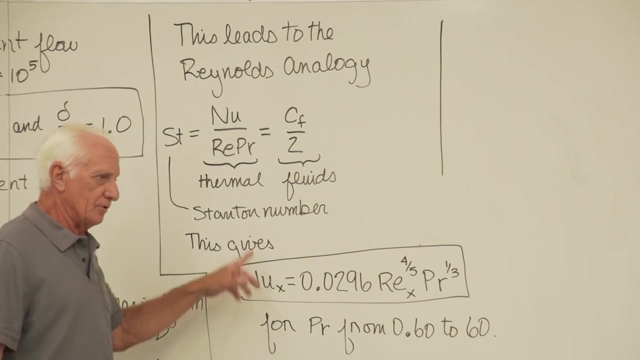 So this guy came by modifying this thing for property variations. Now it's good for Prandtl number from six-tenths to 60.. Okay, so that's the range this equation is good for. What does that replace? Now here's a Nusselt, the local Nusselt number for turbulent flow. 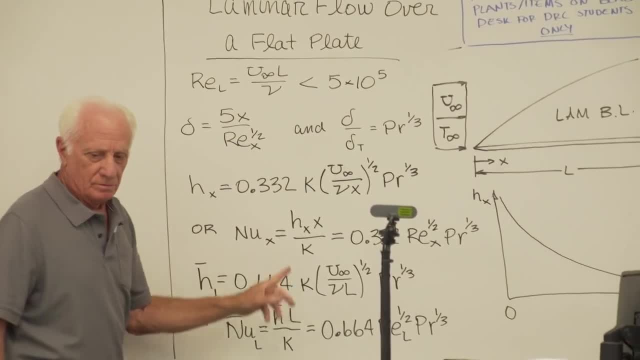 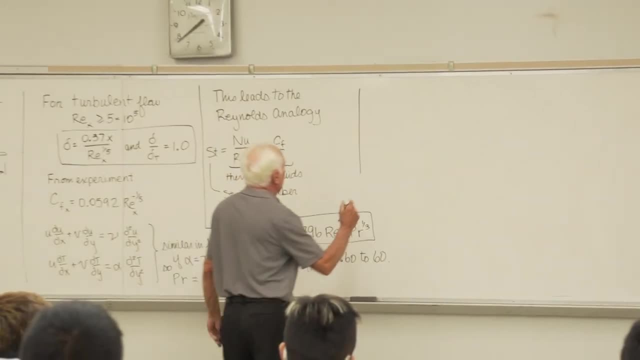 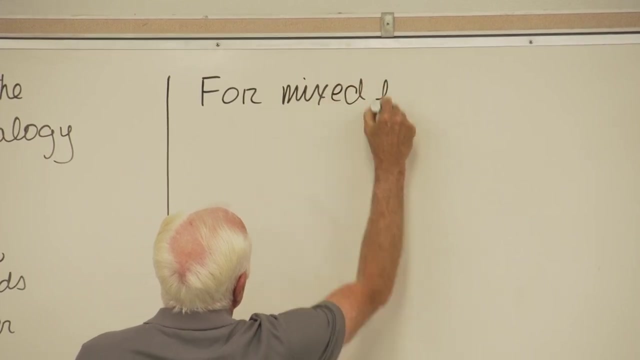 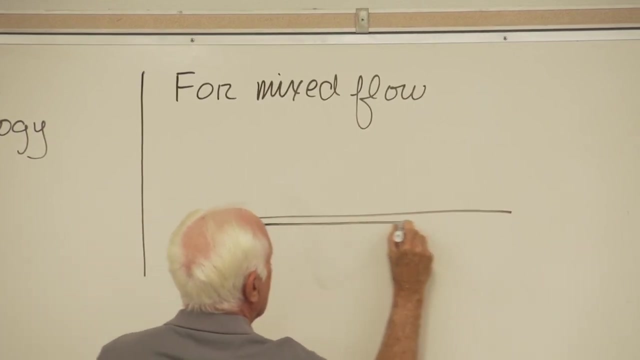 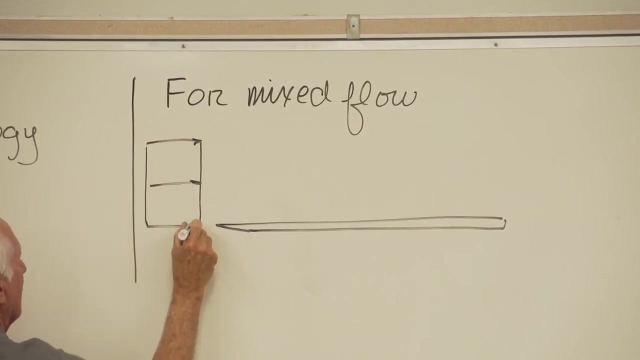 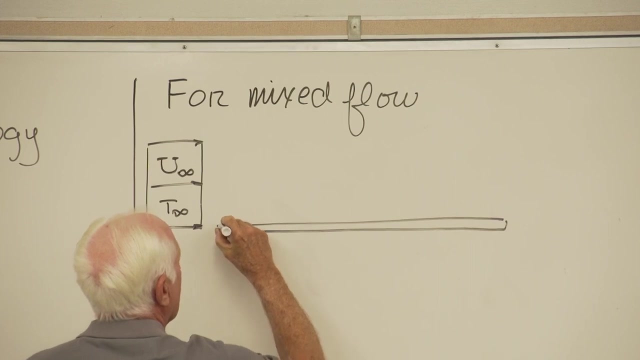 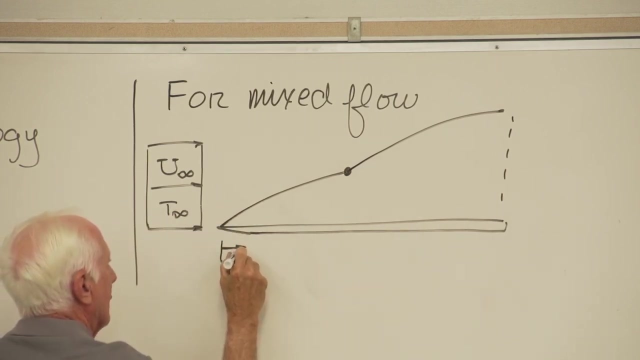 Here's the local Nusselt number For laminar flow. Okay, we got that guy boxed in. Okay, Now for mixed flow. Mixed flow looks like this Because shootresh is positive, therefore, At the leading edge, Fx is still true. 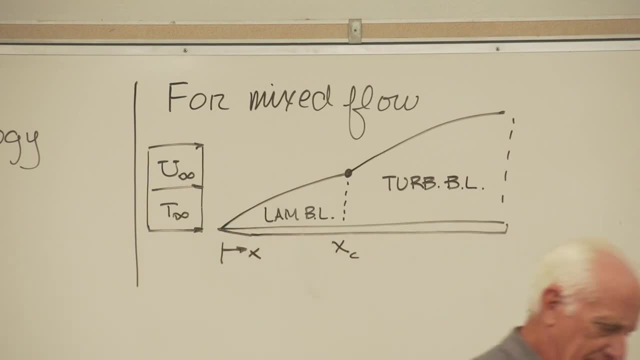 Now significant equals 0, because it's still false, because it's still Unless. So the flow starts out at the leading edge. Thus, So the flow starts out at the leading edge. X equals 0, zero as laminar. Then, as we go down the plate, 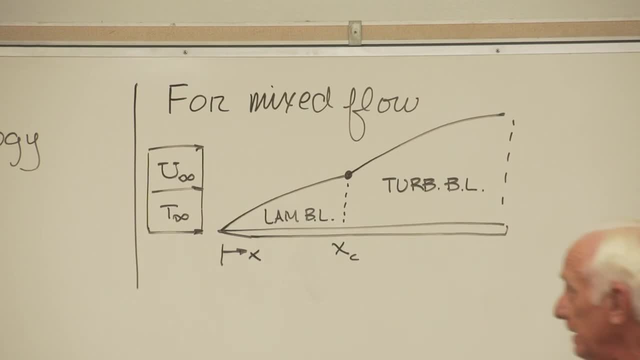 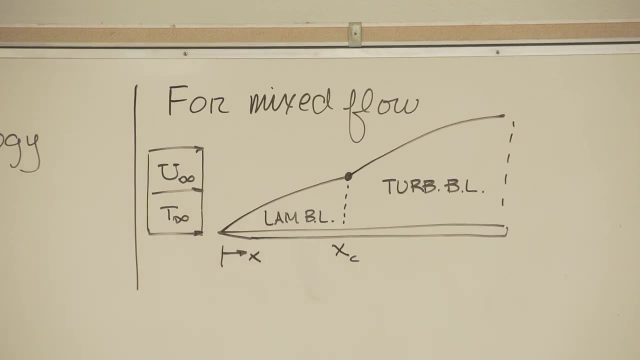 if we get to the point where the Reynolds number is equal to five times 10, to the fifth, the flow transits to turbulent. That's called a mixed boundary layer: part laminar, part turbulent. Well, the same old thing. we want to find h. this is heat transfer class. 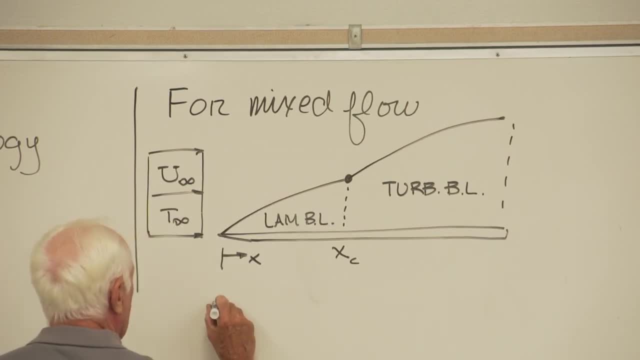 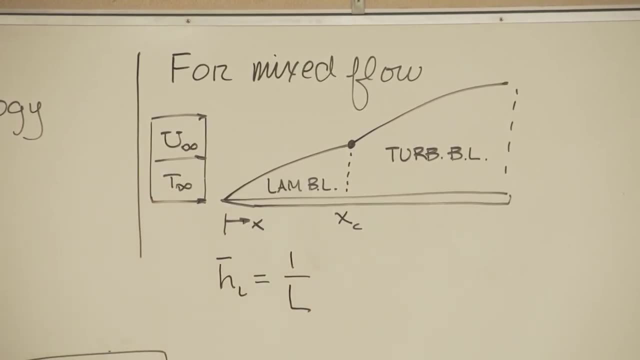 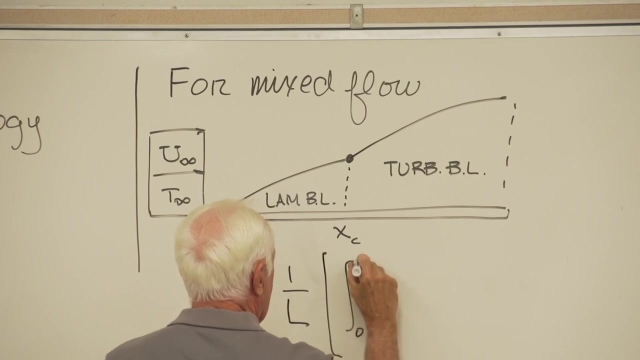 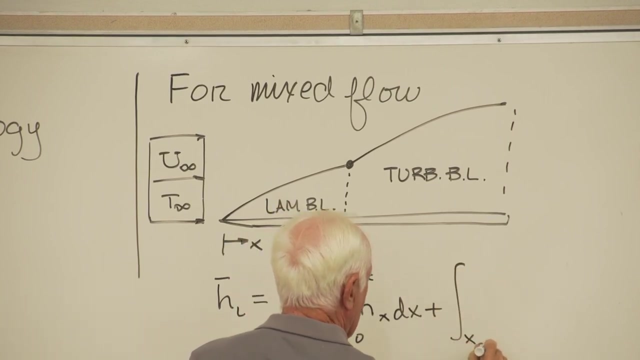 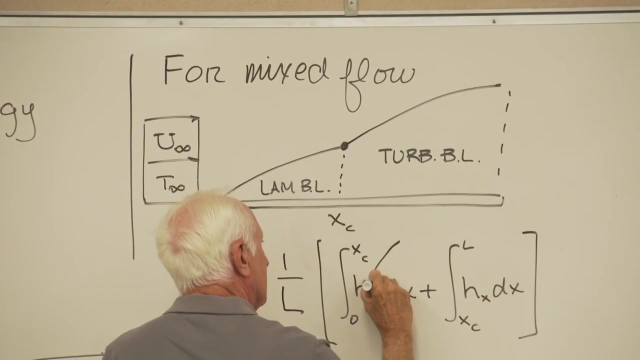 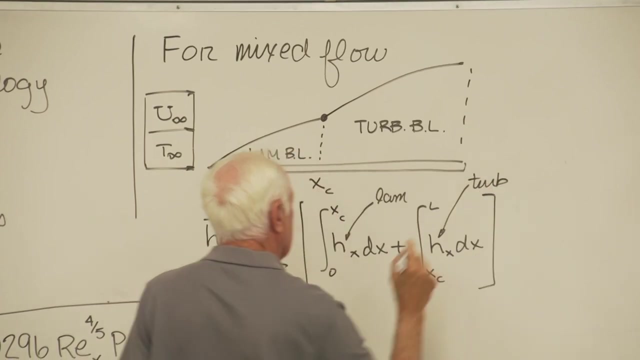 So we want to find h. So h-bar L, we have to get the integrated average value over the whole plate length L. The h-x here is of course the laminar h-x. The h-x here is of course, the turbulent h-x. 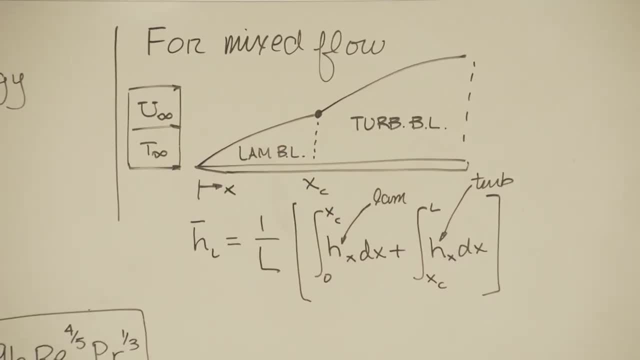 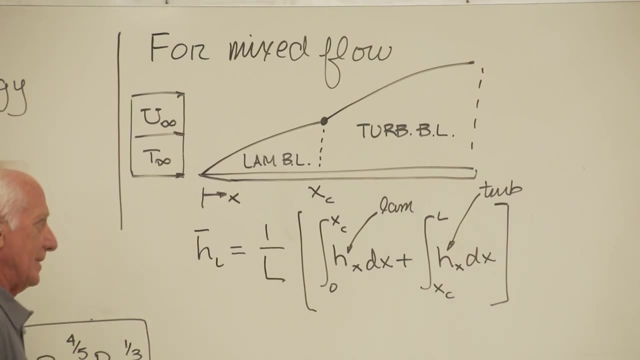 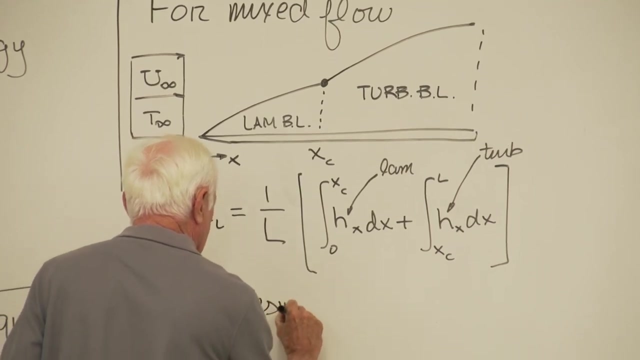 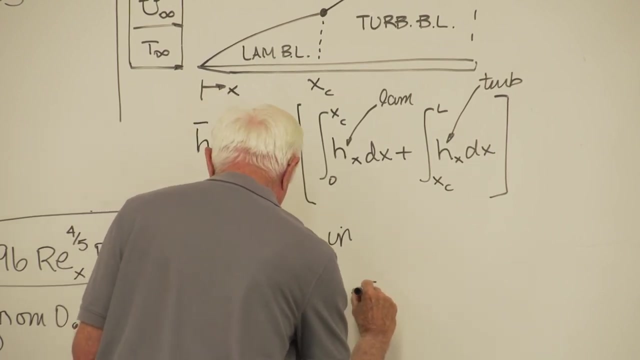 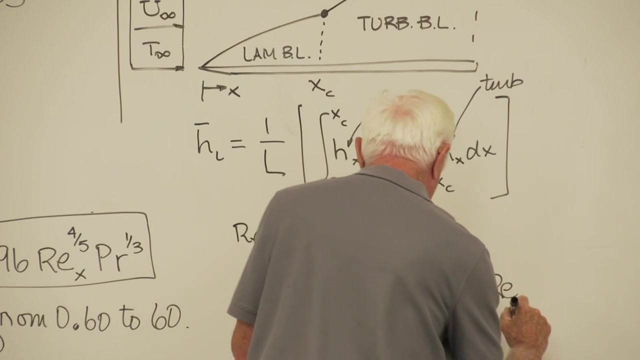 So you put this guy for h-x, for turbulent, there and you put over there the h-x here and you carry out the integration and we jump down to the result. So that's the whole thing. Now we're going to look at this. 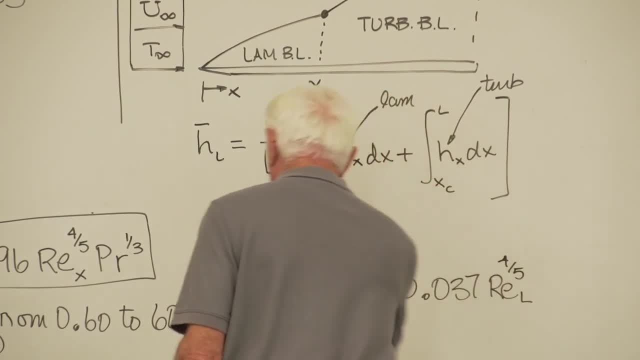 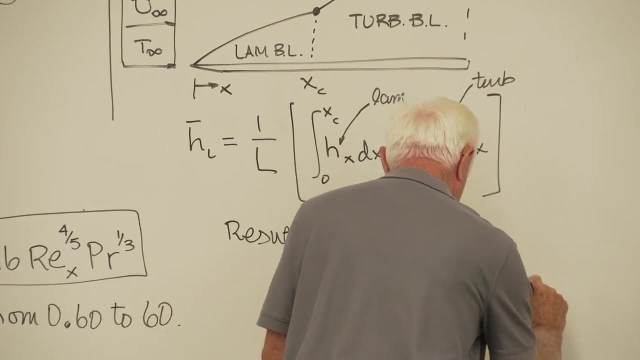 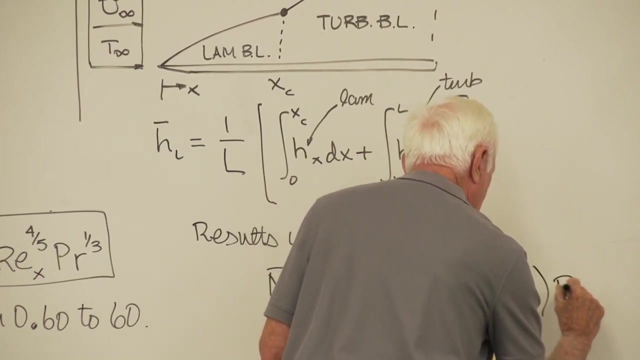 for a moment, and then we'll look at this for a moment. So that's the logic of it. That's the logic of it. That's the logic of it. We all know all the laws. We know all the laws. We know the laws. 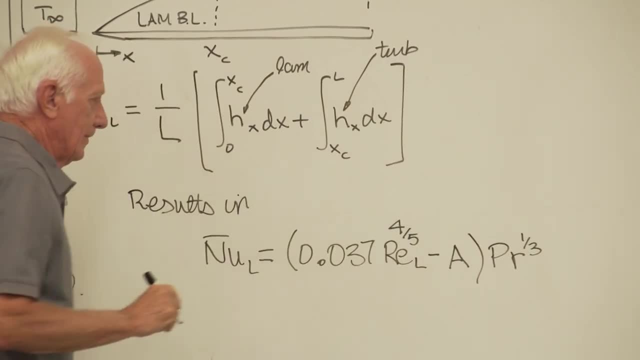 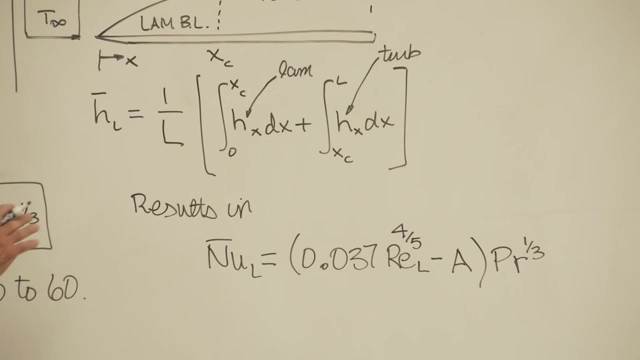 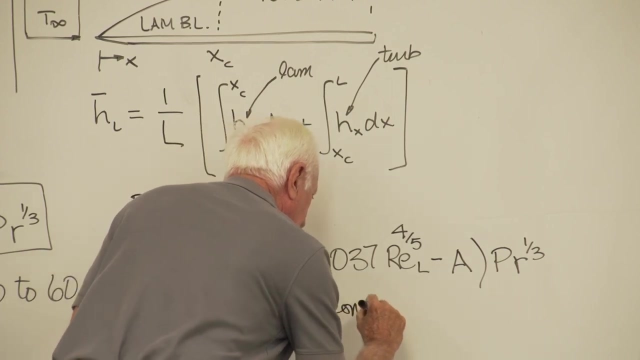 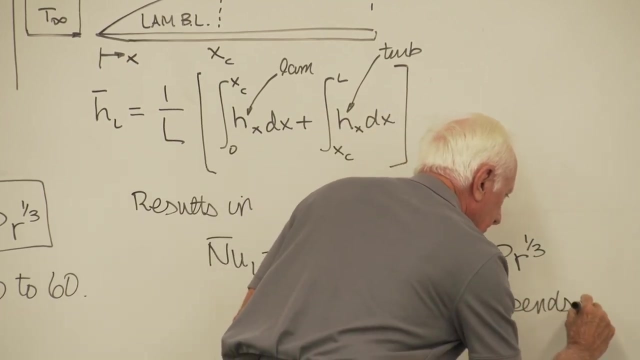 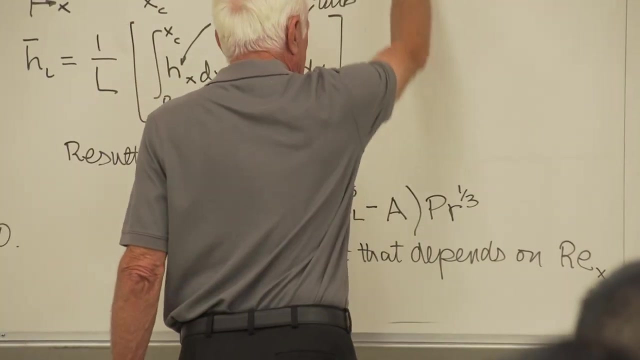 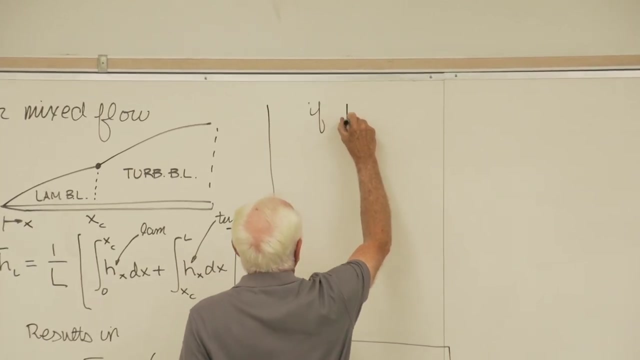 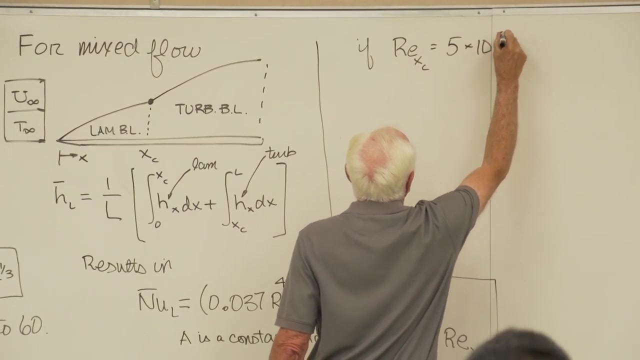 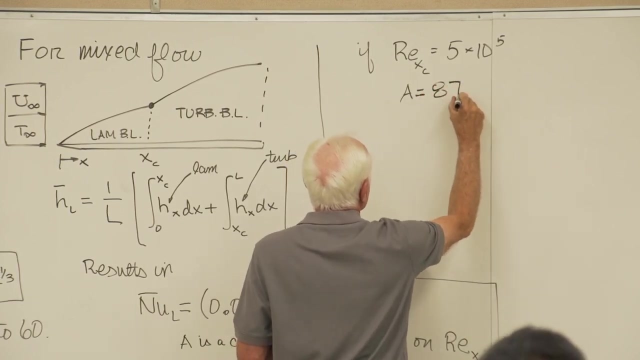 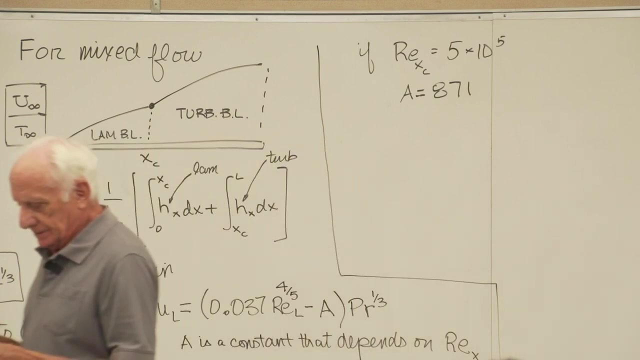 it results when you're all done with the integration and clean it up. it results in that Now that A, he says, is a constant, What he's saying is that constant A depends on what the critical Reynolds number is for transition from the lambda to the determinant. 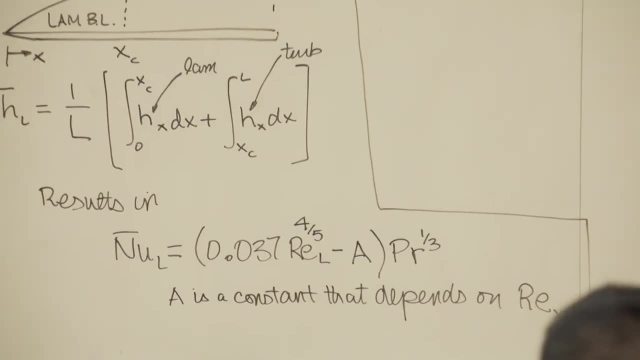 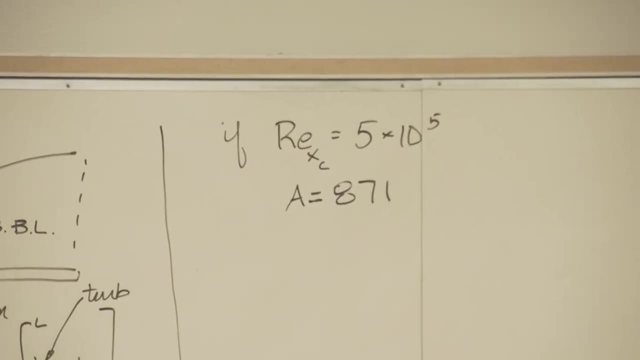 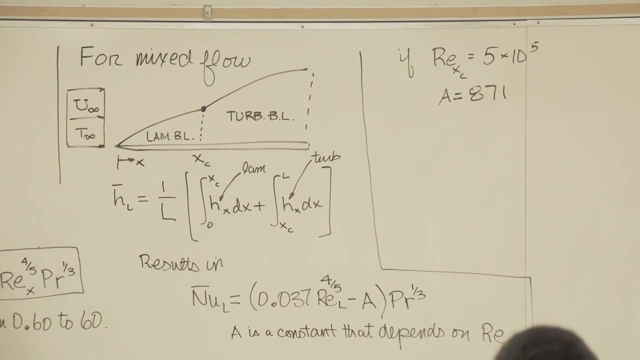 We use 500,000.. The textbook for homework, for quizzes or exams, we use 500,000.. But in the real world it could be different. That 5 times 10 to the 5th depends on the approach. 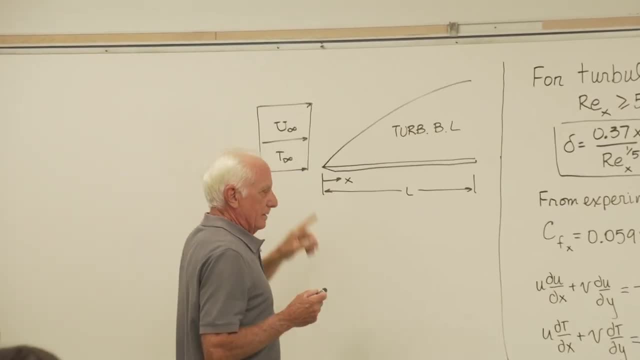 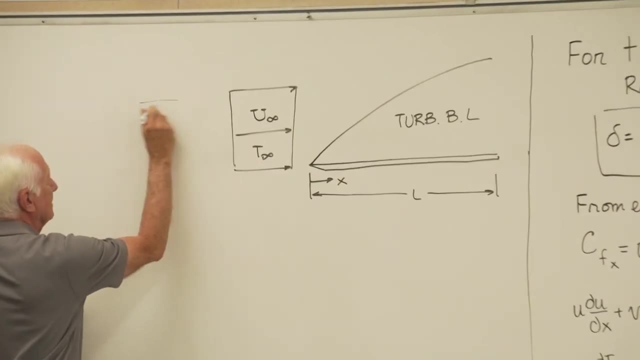 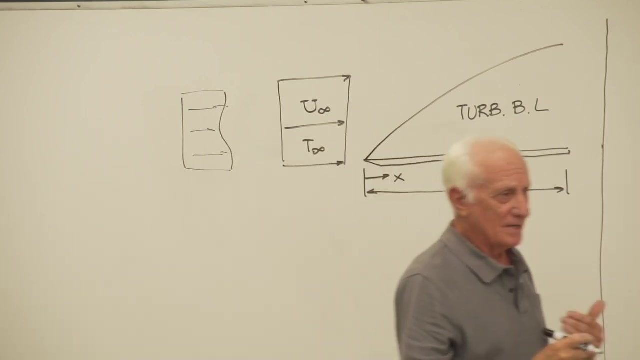 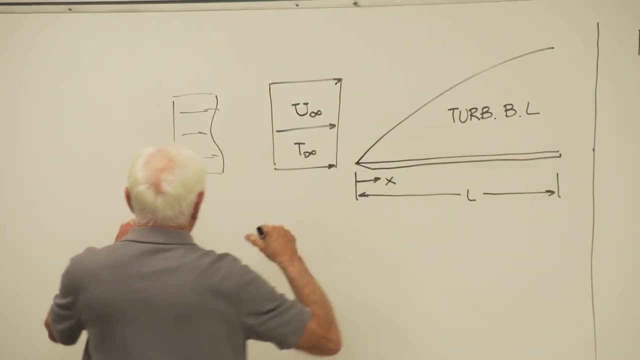 the approaching stream, It better be. you can see here, it can't be something like this. No, that flow is not going to transition 500,000. if that's the approaching free stream, It has to be uniform. uniform Streamlines are perfectly horizontal. 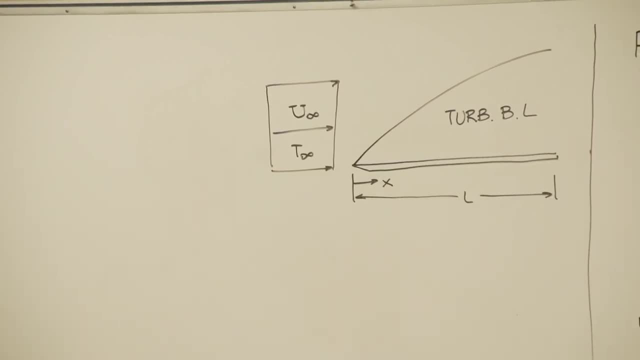 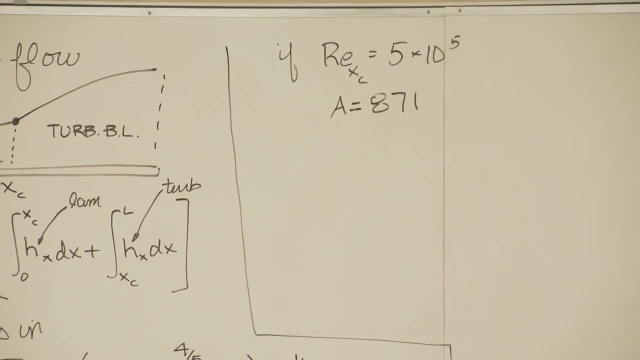 under all perfect conditions. Then the critical Reynolds number is 5 times 10 to the 5th, So we don't need to worry about that. in this class The textbook always uses 5 times 10 to the 5th. That's okay. 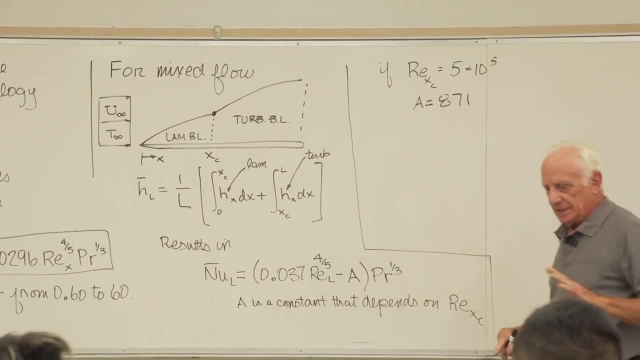 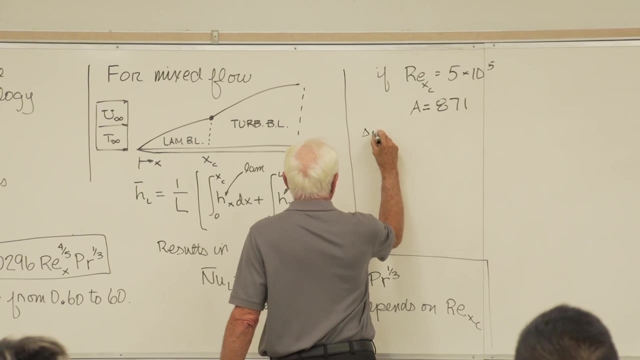 If it's not 5 times 10 to the 5th, then that A changes. He tells you what to do in the textbook, but we're not concerned with that. In our case, A is 871.. So we have no salt bar L. 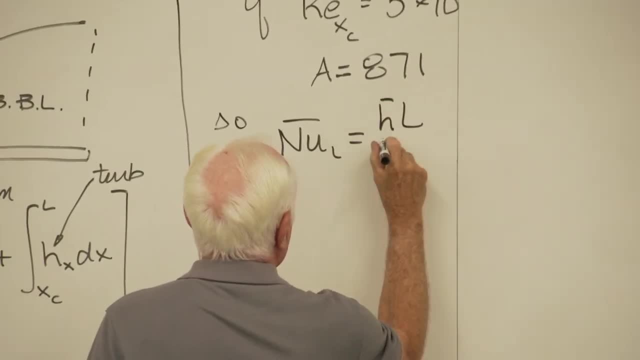 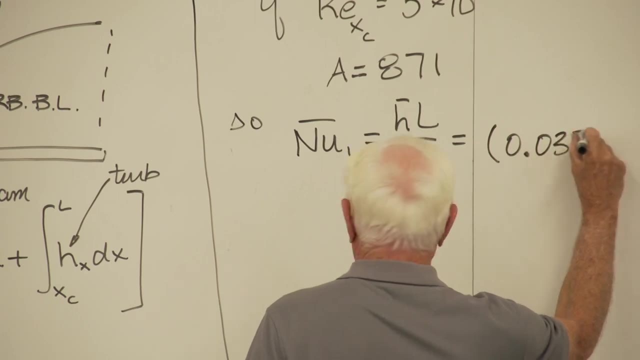 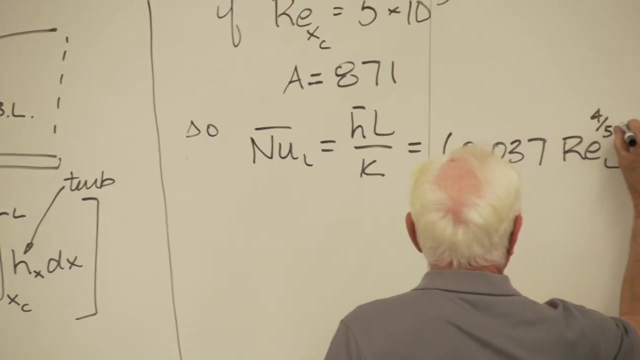 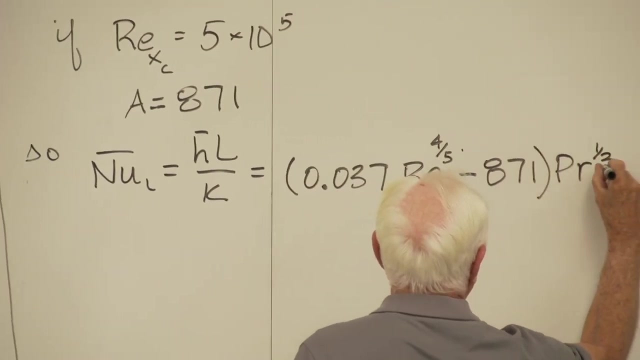 Equal H bar L over K 037.. Reynolds: L to the 4th, Minus 871.. Crandle to the 1- 3rd. That's how we get the average H. For next time let's flow. 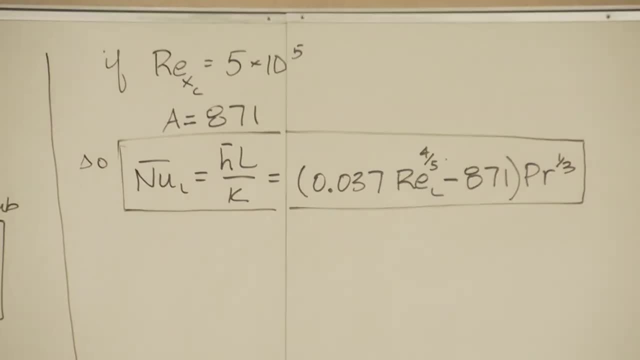 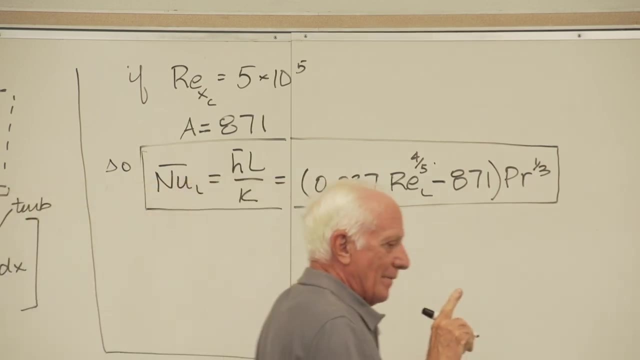 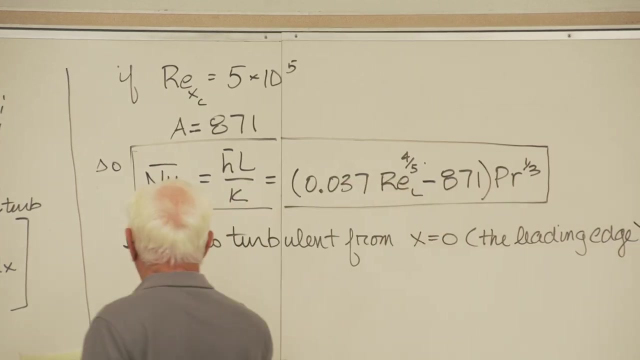 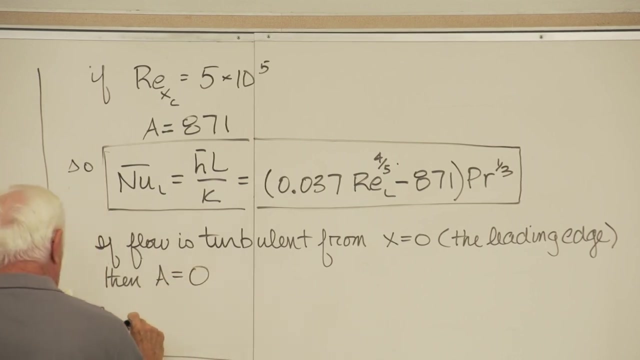 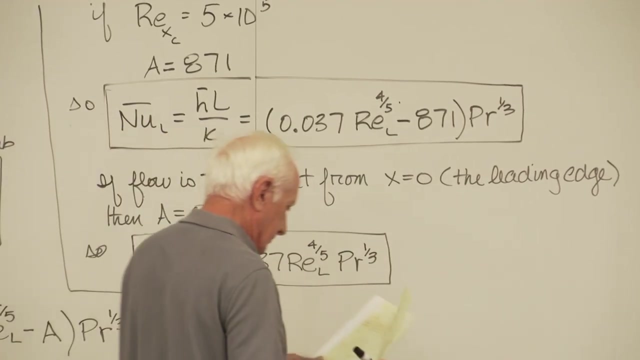 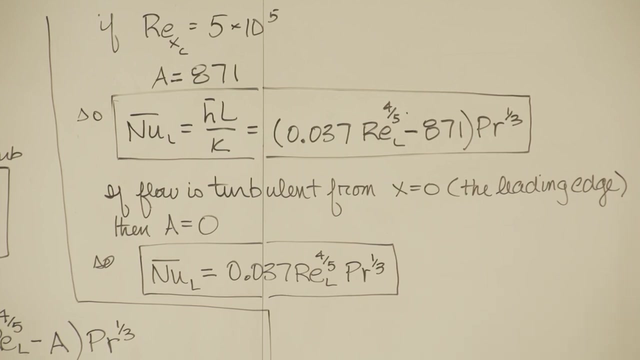 Let's flow. Now he also says: if the flow is turbulent from the leading edge, let's say we'll do the symmetric force, then A equals zero. So we get this And we get this as the spin of the Okay. So that is the average value of the Nusselt number. 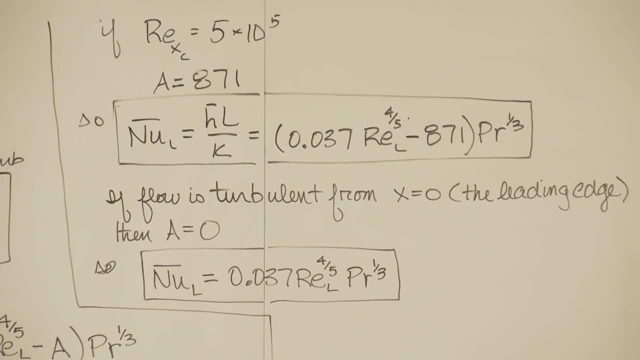 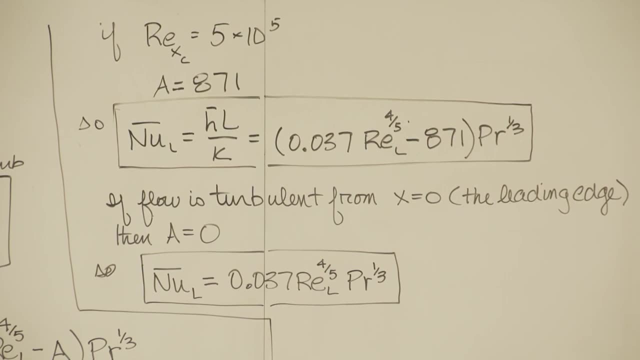 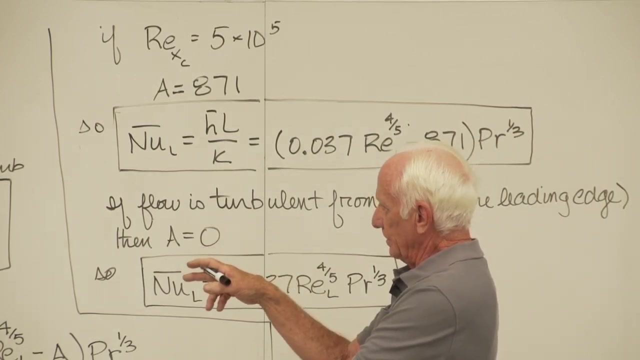 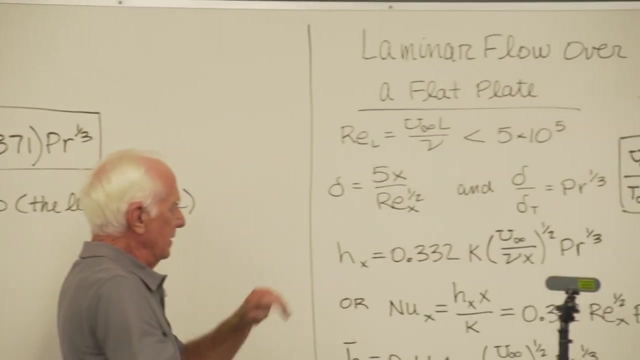 which is of course the average value of H, if the flow starts out turbulent from the leading edge. So these boxed equations on the board right now are added to these equations over here for laminar flow: Delta, delta, t, H, sub, x, H, bar. 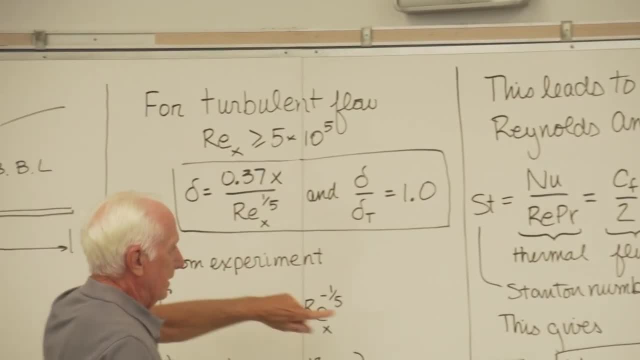 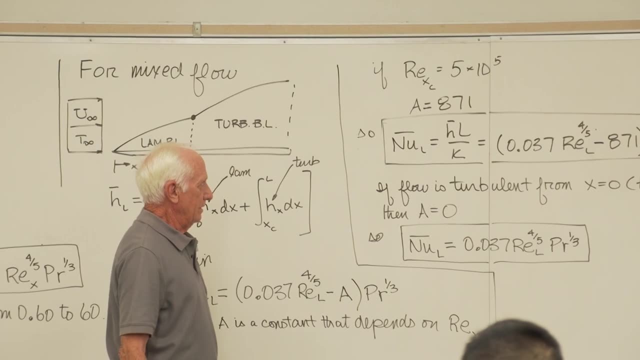 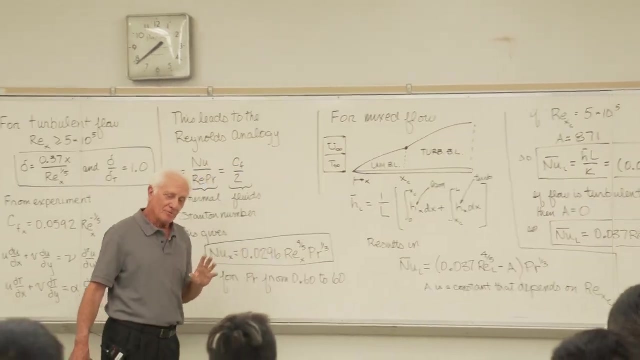 Delta delta t H x, H bar. If it's mixed flow, H bar. The first thing you do in a problem, of course, is you find the Reynolds number At the end of the plate, Or you can find x of c. 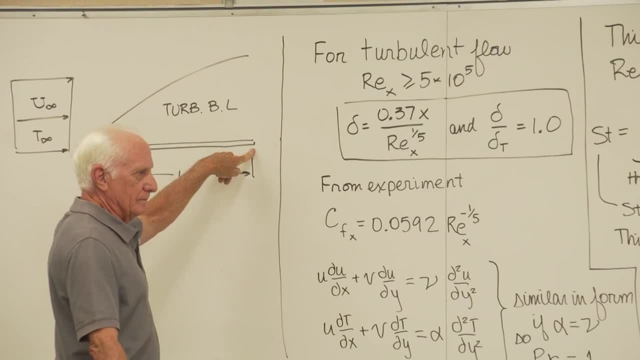 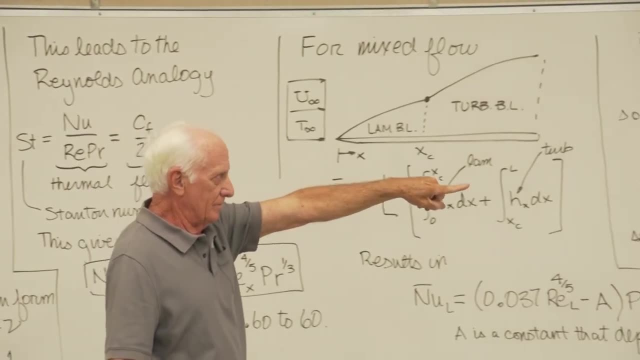 But let's just say you find the Reynolds number at the end of the plate. If it's less than 5 times 10 to the 5th, you've got all laminar flow. Life is very straightforward. What do you want to find? 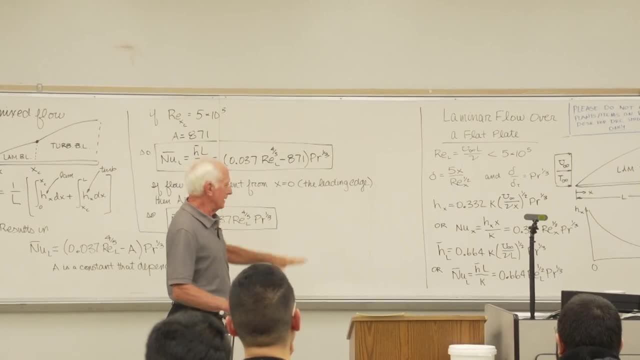 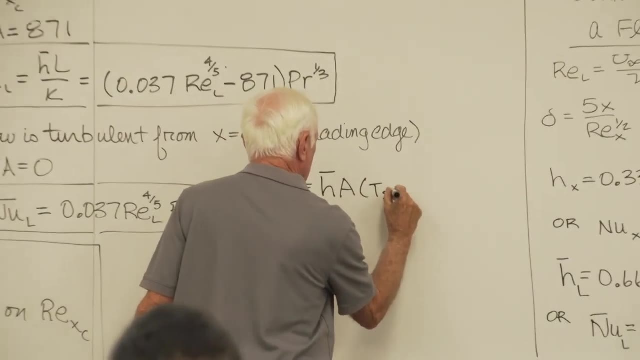 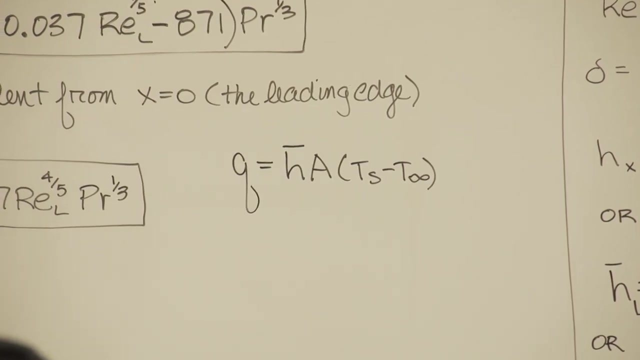 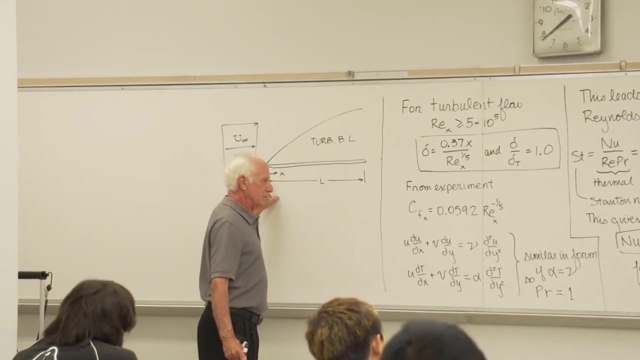 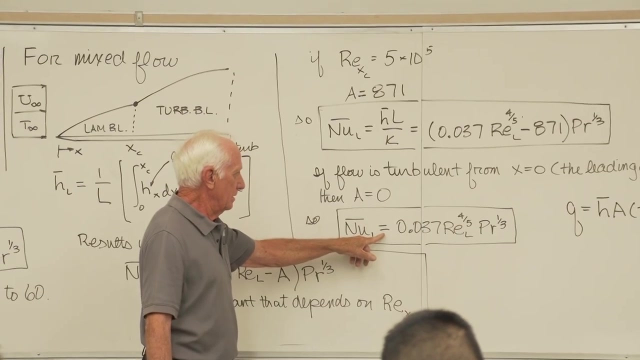 I want to find the heat transfer over the whole plate If the flow starts out turbulent from the leading edge. And I want to find the heat transfer from the plate, I need an H bar for turbulent flow. There it is. Put that H bar in here. 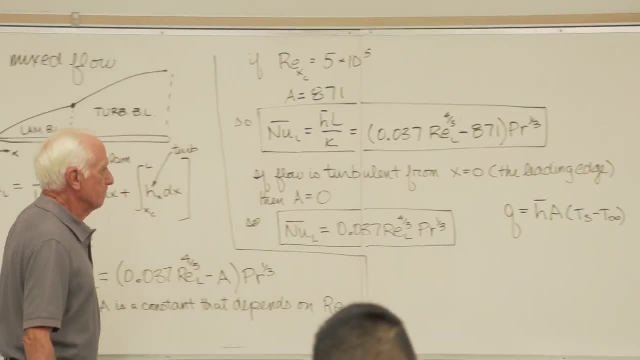 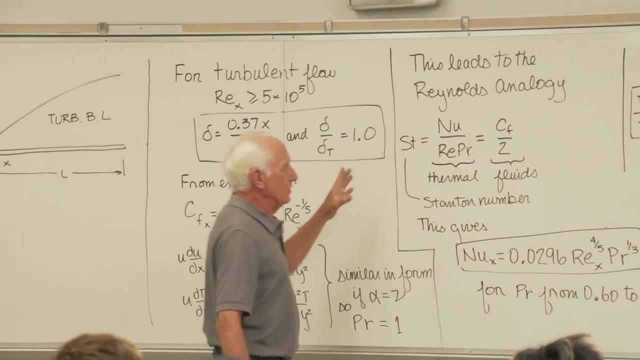 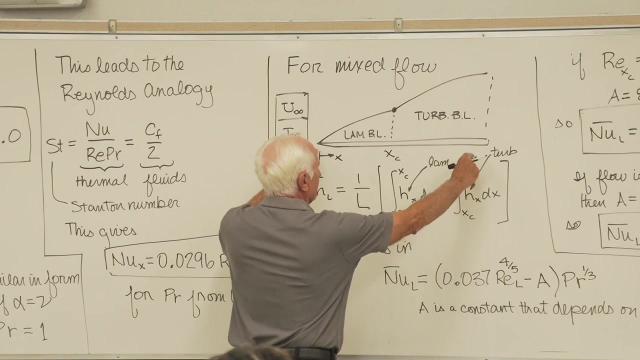 End of problem. Got it Now. the problem says the problem turns out mixed flow. Reynolds number at the end of the plate is turbulent, Greater than 5 times 10 to the 5th. Find out what x of c is. 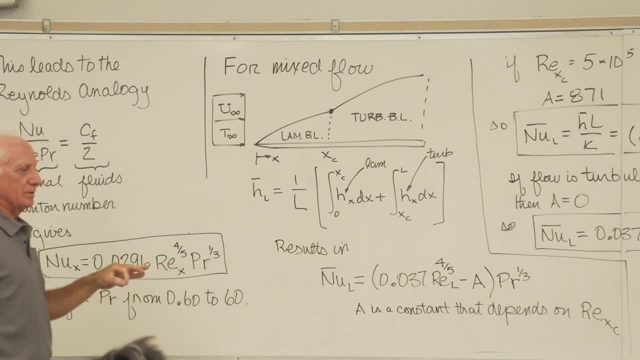 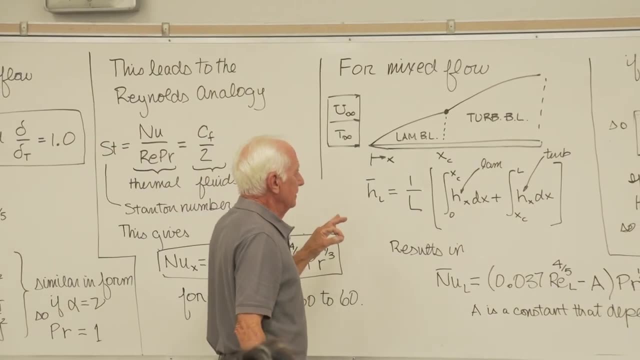 How do you find x of c? Equate the Reynolds number to 500,000.. Solve for x. That gives you x of c. So if I want to find the heat transfer over the whole plate, find the heat transfer over the whole plate length. 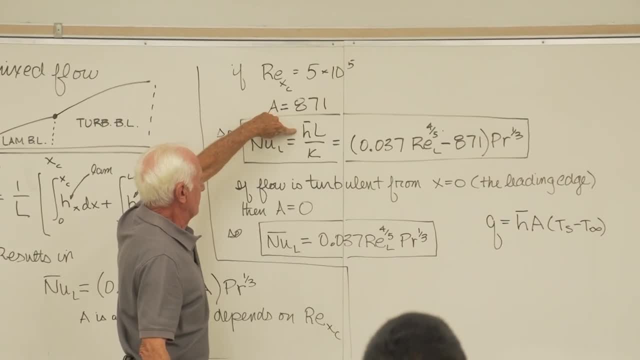 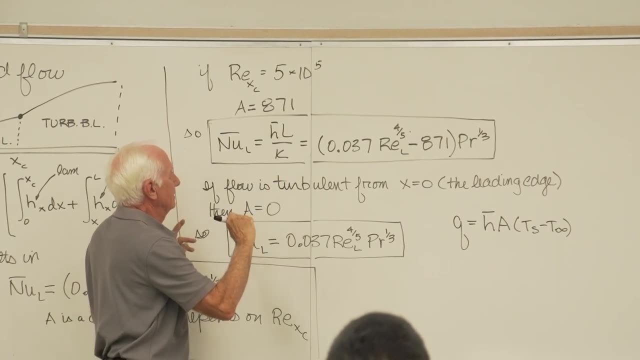 Right here. There it is H bar. Some people- I hate to mess this up, but they'll put an H bar subscript L. It gets to be too much in there, So H bar L. Where do you put the H bar? 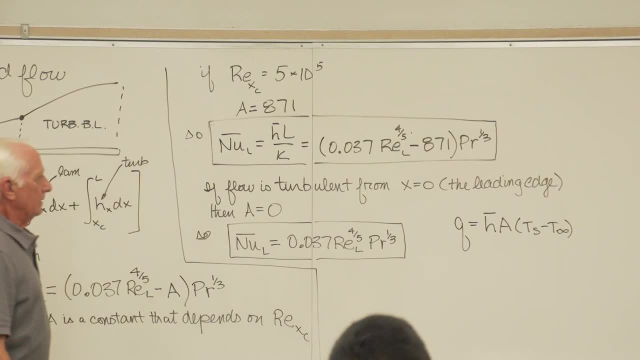 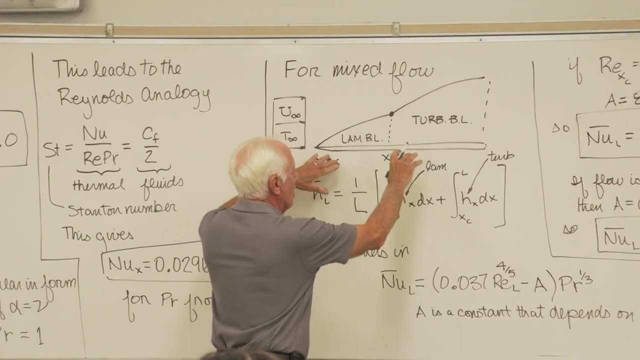 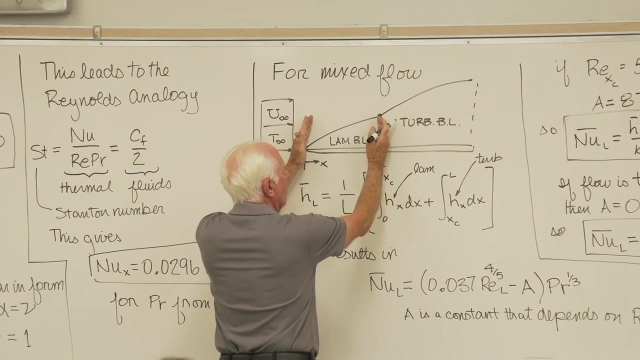 In here, Got it. If someone asks you how much heat is transferred Over the laminar part of this mixed flow from here to here, What do I do? Okay, I find H bar for the laminar boundary layer. Okay, 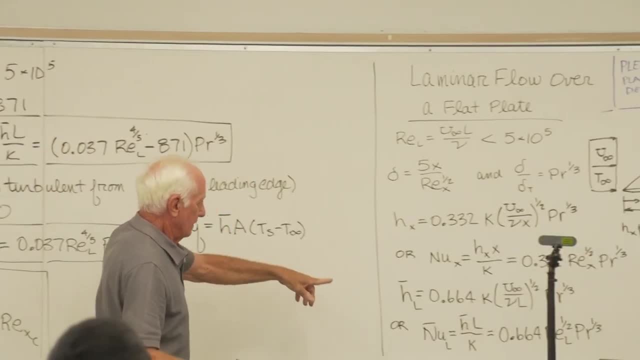 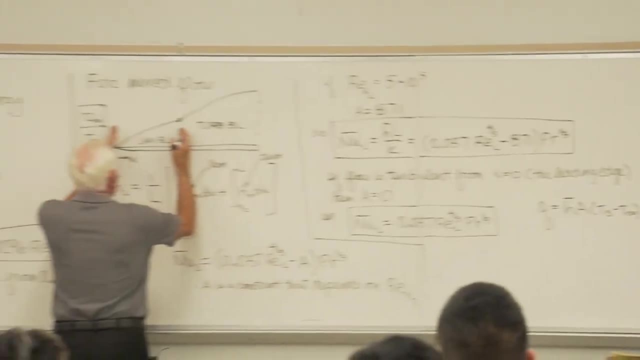 There, it is over there. Okay, What do I put in for L in that equation? Oh, you don't put in L the plate length. You put the L where my right hand is. My right hand is where x of c is. 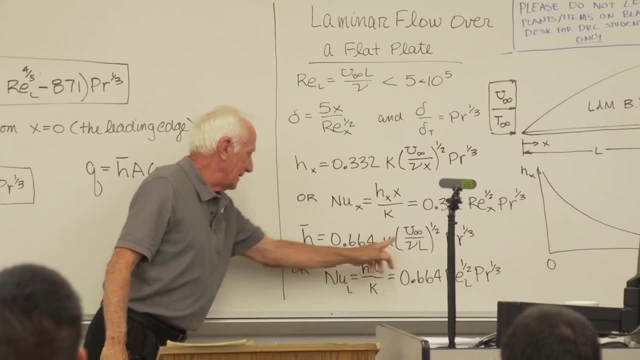 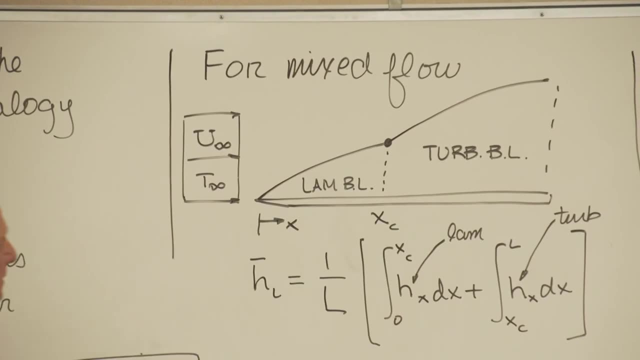 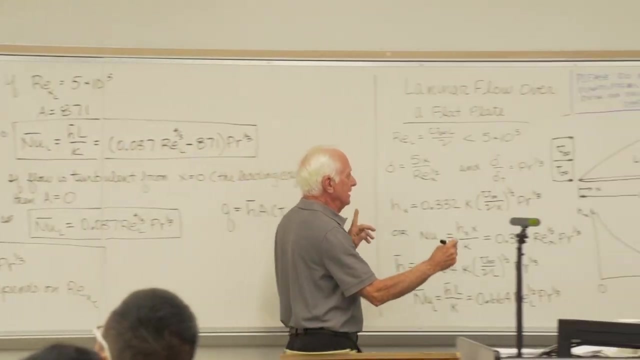 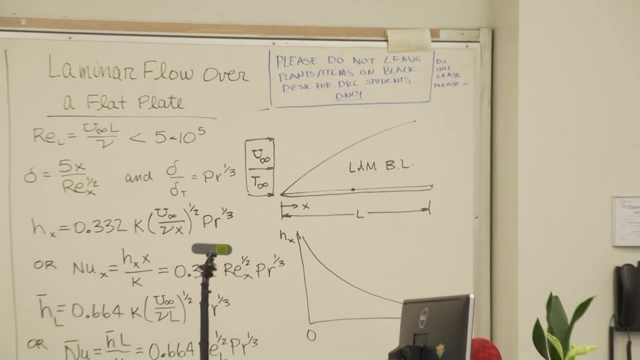 I put x of c here, That gives me the H bar over the laminar part of the boundary layer. What if someone says: I want to find the local heat flux? where x equal L over two, where the black dot is, I want to find the local heat flux. 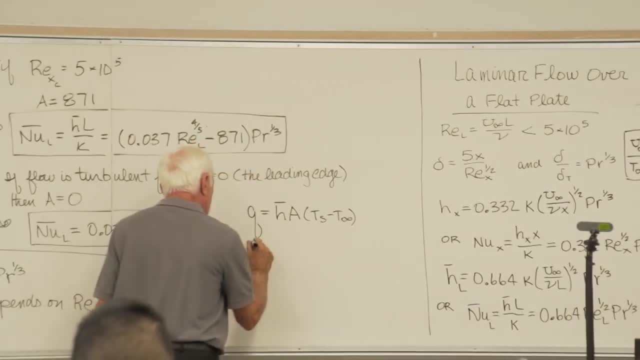 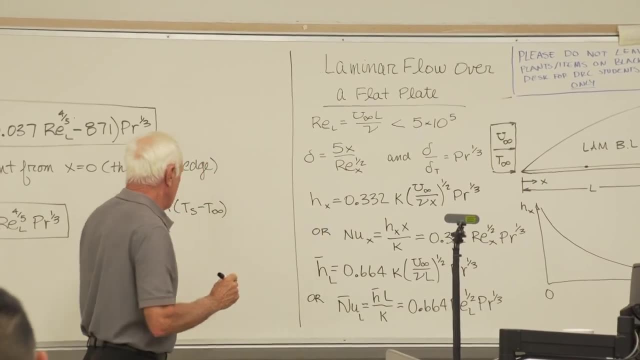 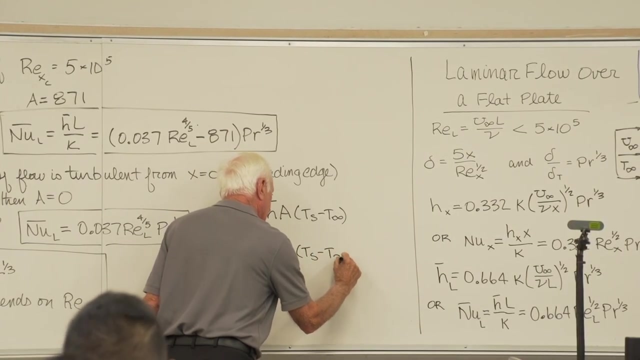 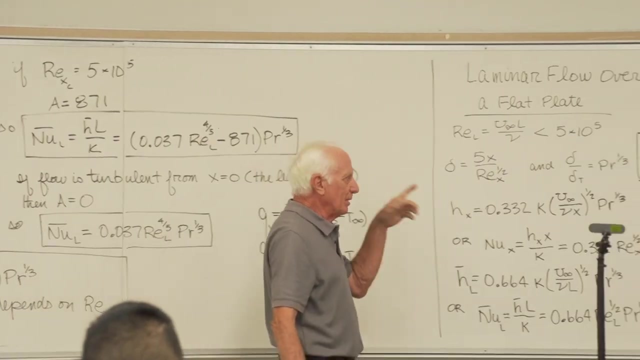 Don't forget the word. heat flux means Q, double prime, Local heat flux. I need Hx, the local convection coefficient. I don't put the area in because it says heat flux. What if somebody says I want to find the local heat flux at the end of the plate here? 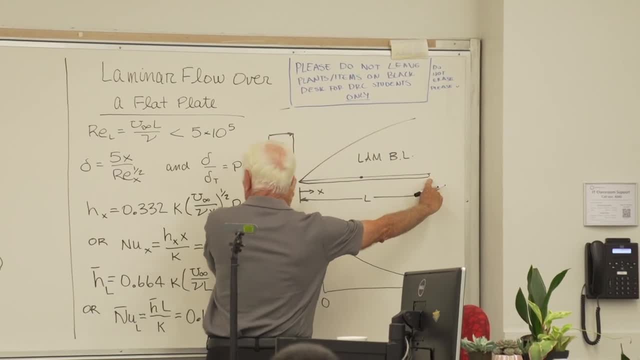 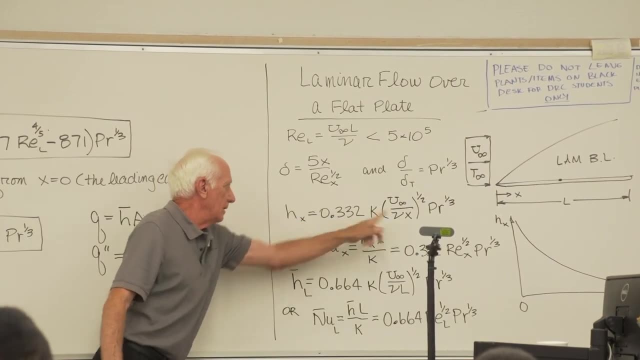 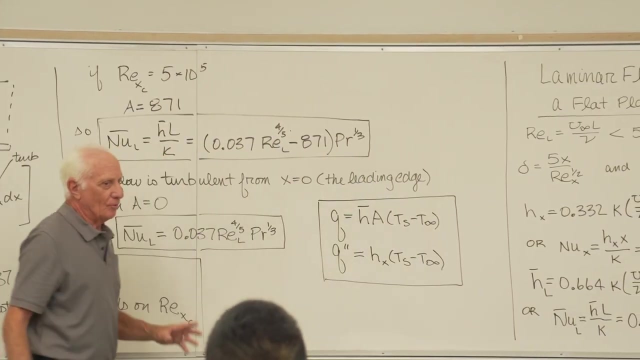 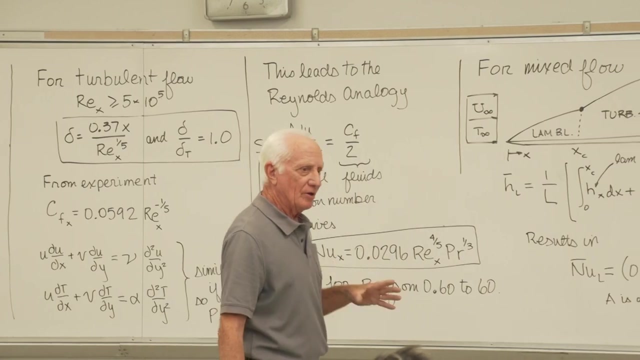 Fine, Where's my right hand? X equal L. Put L in there. Find H right here. Put L in there. There, it is Very simple. As I said before, once you get H, life becomes much easier. All the work is done in getting the right value of H. 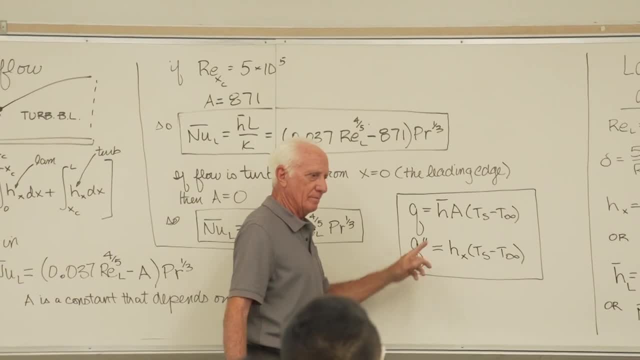 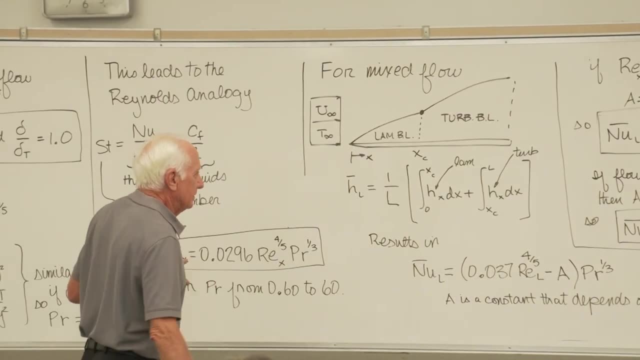 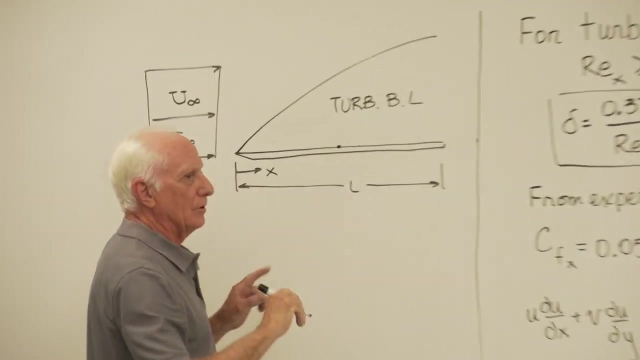 Qs fall out once you get to H- Either him or him. Again, turbulent flow. Someone says: I want to find the local heat flux at x equal L over two Local subscript x. right here, What do you put in for x? 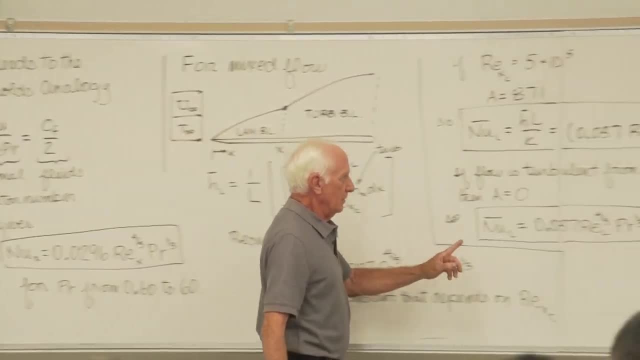 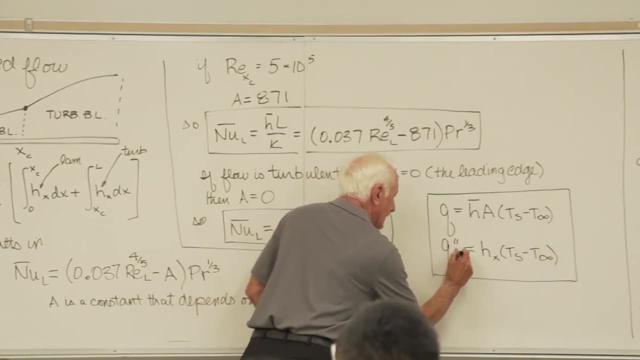 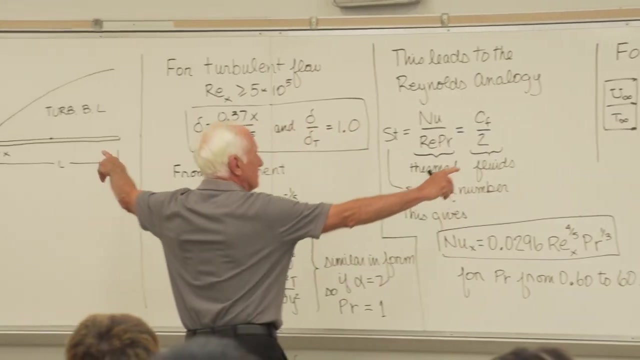 L over two, Got it. What do you do then? Put it in here and get the local heat flux. Sometimes you can put an x here That just indicates at that particular x location. Okay, What's the difference in these two guys? 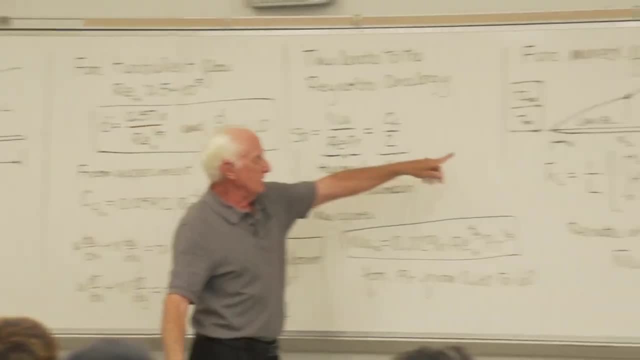 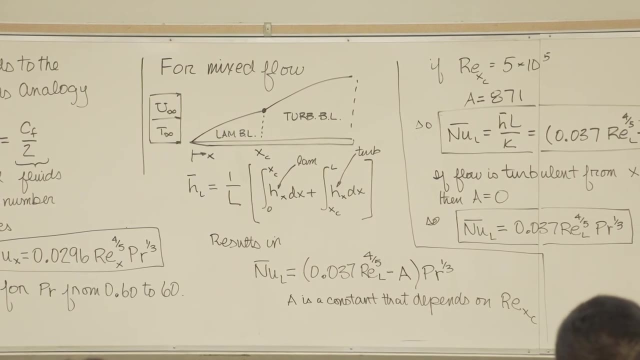 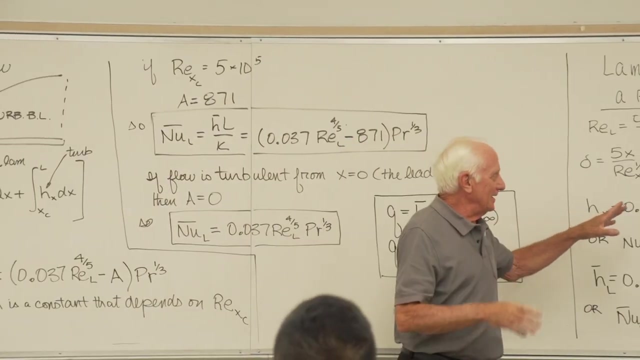 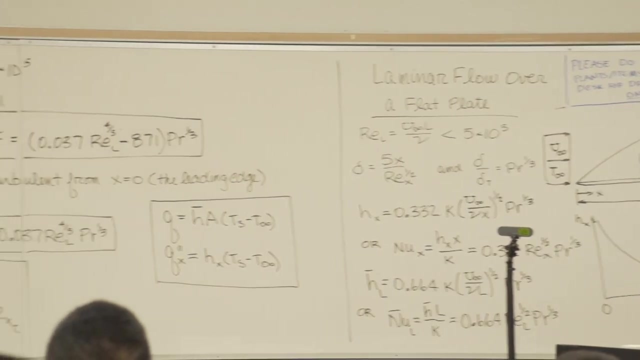 How come he starts out turbulent from the leading edge but he starts out laminar? Well, you've got to read the words real carefully. You won't find a totally laminar boundary layer. a lot in the real world It's hard to get. 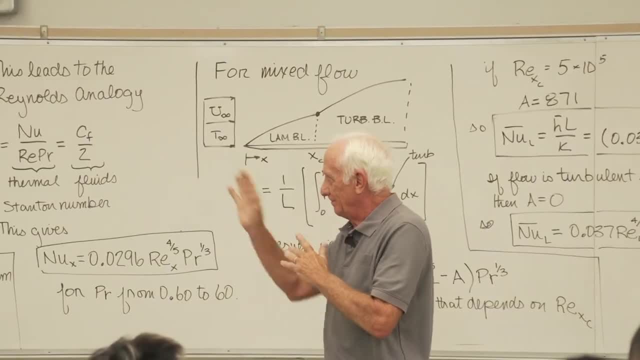 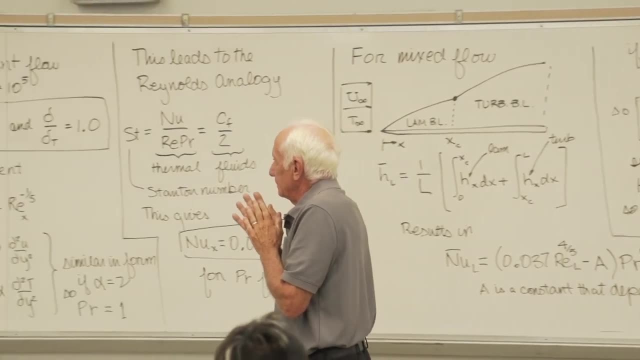 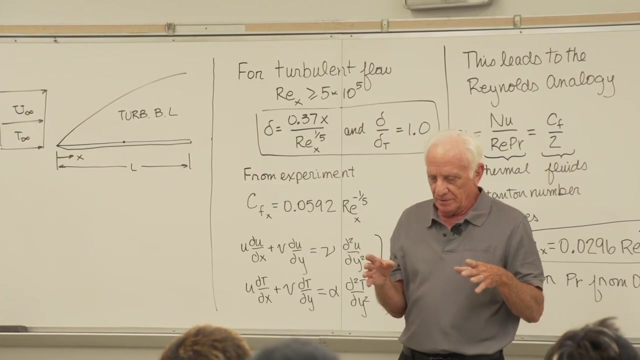 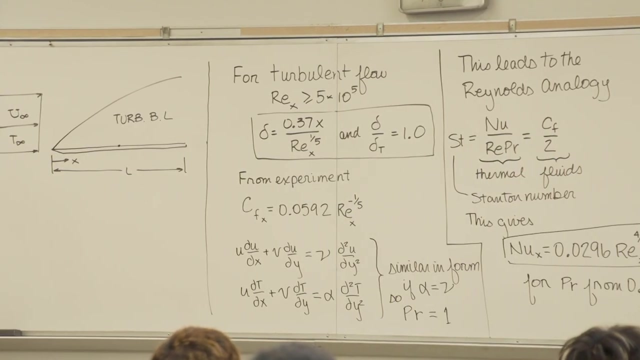 It's hard to get because the flow approaching the plate is not always as nice as you'd like it to be. So we had the problem. We worked in class a couple of class meetings ago, The tractor-trailer truck with the trailer, And the problem said in words: it said: find the heat transfer or find the temperature at the top of the truck. 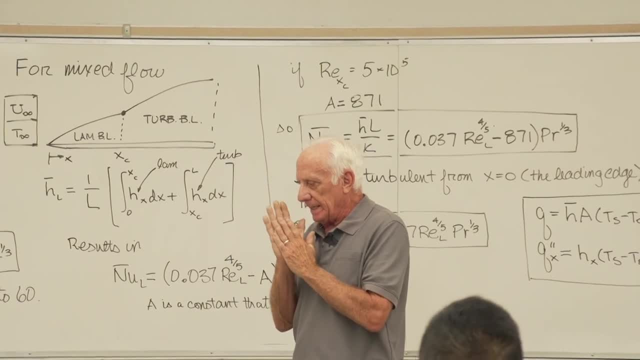 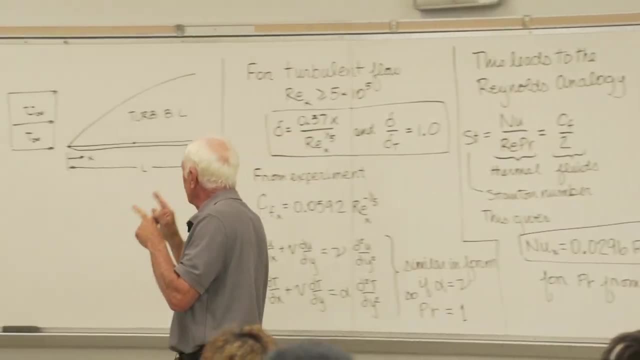 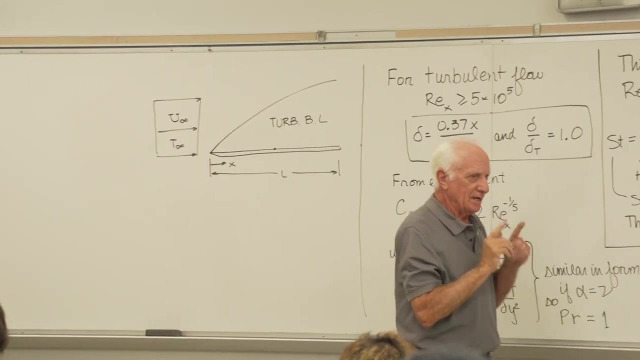 Assuming the flow, Assuming the flow is turbulent from the leading edge of the trailer body. Okay, So he told you that. He told He said: assume it's turbulent boundary layer from the leading edge of the trailer body. If the problem says nothing like that, then you do it this way. 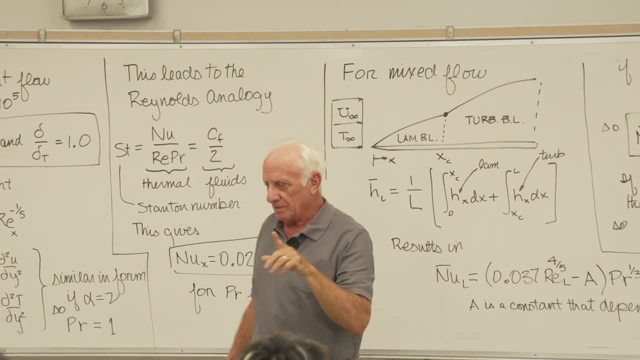 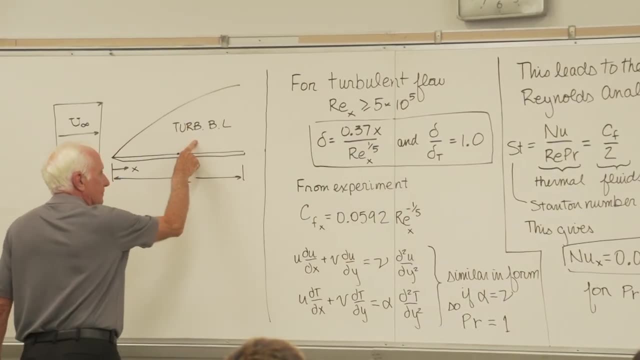 Assume it starts out laminar. If you see the magic words in the problem or an exam that the flow starts out turbulent from the leading edge, you do this guy. So look for those words in the homework problems, in the textbook or in the exam or quiz, whatever. 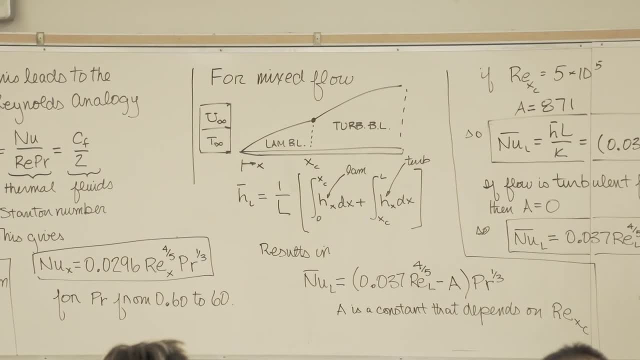 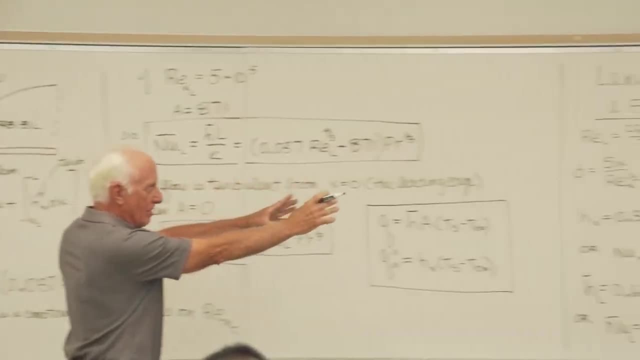 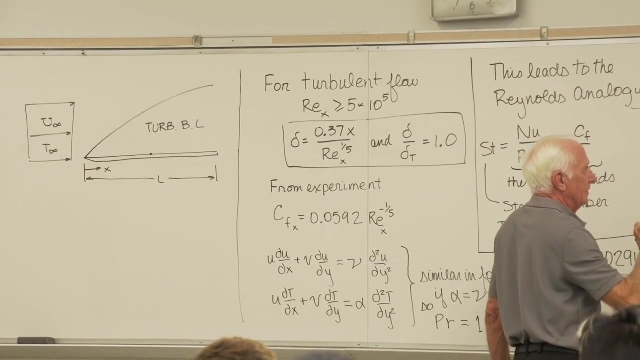 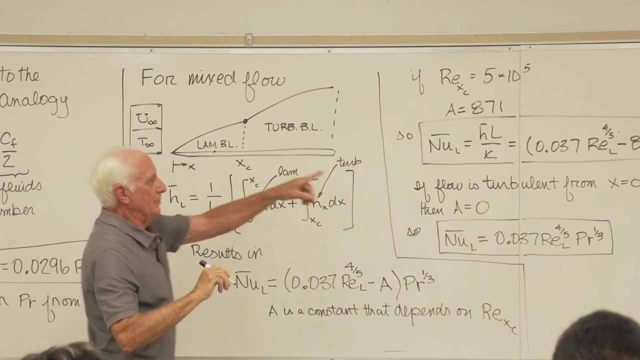 Look for those words. Okay, So three possibilities: All laminar on the plate, All turbulent on the plate And a mixed flow. So if I want to find the heat flux at that little point, I go to over there and for X, I put in that point right there that X value. 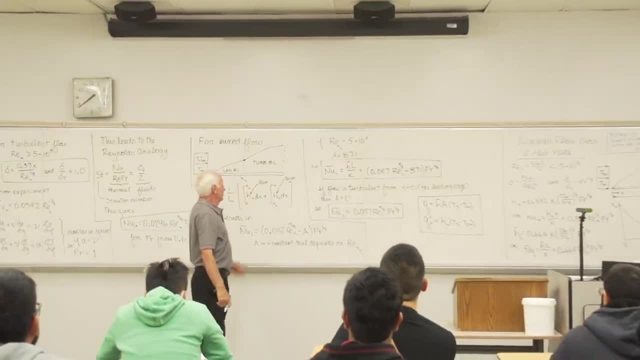 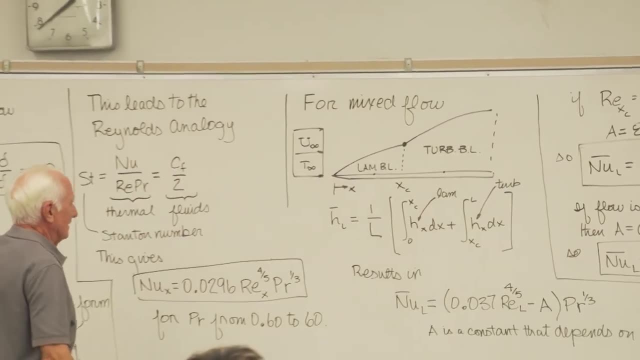 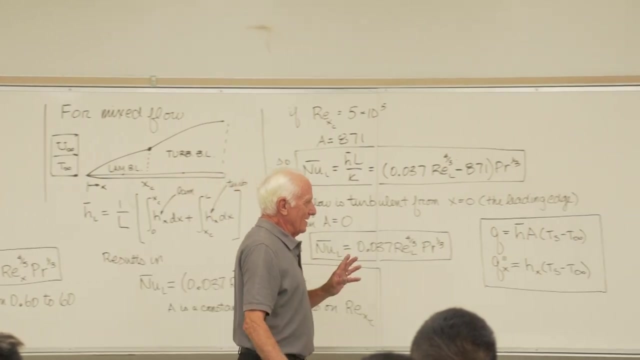 Okay, Turbulent boundary layer. If I say, what's the local heat flux? right here, Turbulent local, right there, There, it is Turbulent local, Turbulent local. So everything in chapter seven Externally. 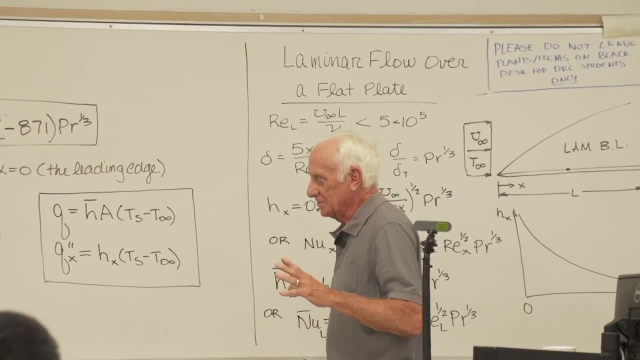 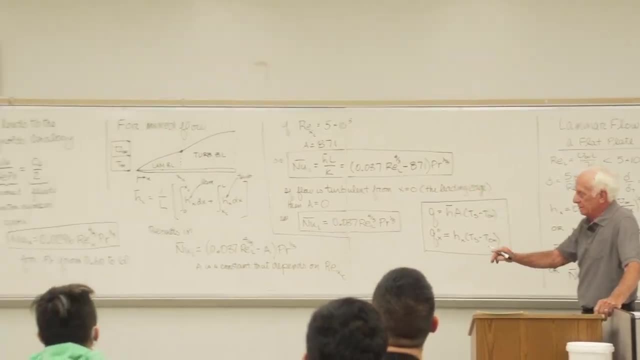 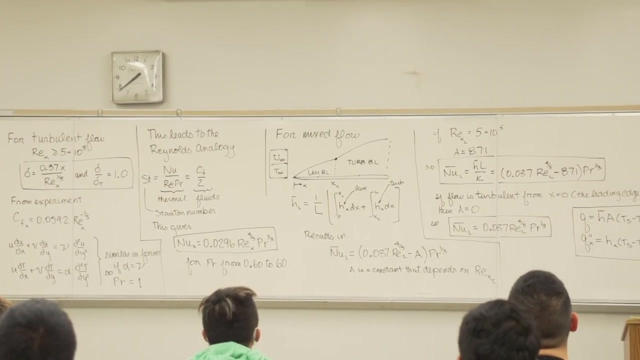 Externally That is useful in solving problems is on the board right now: Laminar, All laminar, All turbulent Mixed flow. Get the right value of H, Maybe. find delta or delta T. Find the local H. Find the average H. 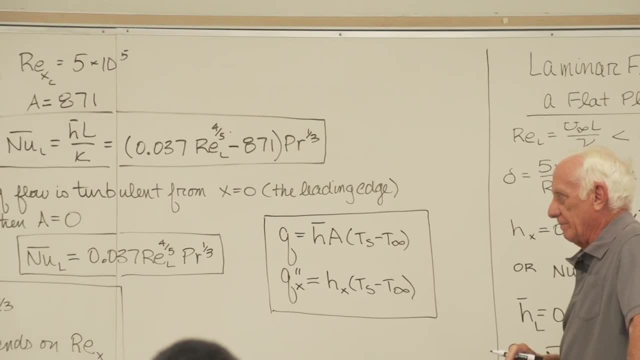 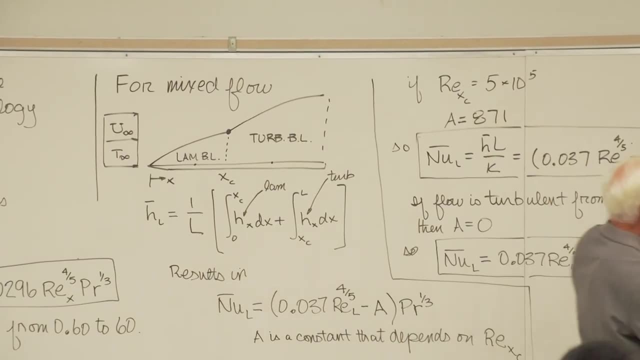 Put them in the equations for Q, Q or Q double prime. That's it for a flat plate. We didn't draw this, but I drew a flat plate. Let's do a picture over there of how H, X varies with X. 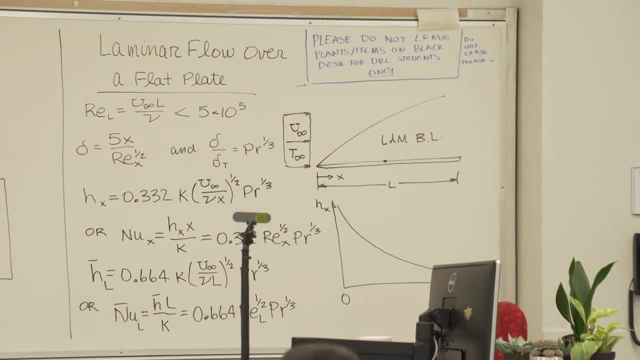 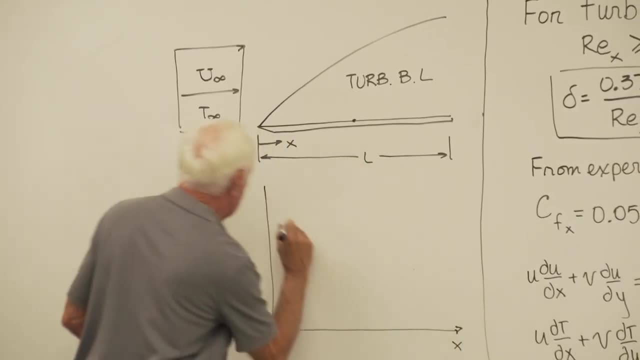 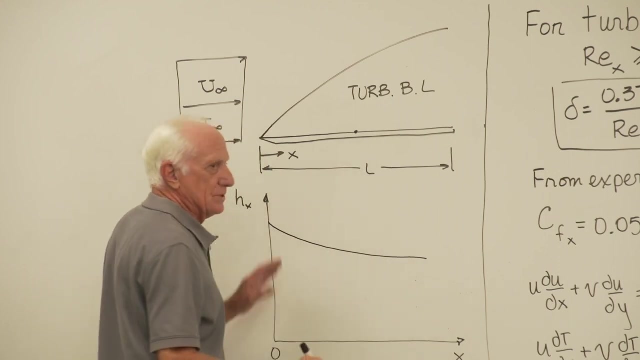 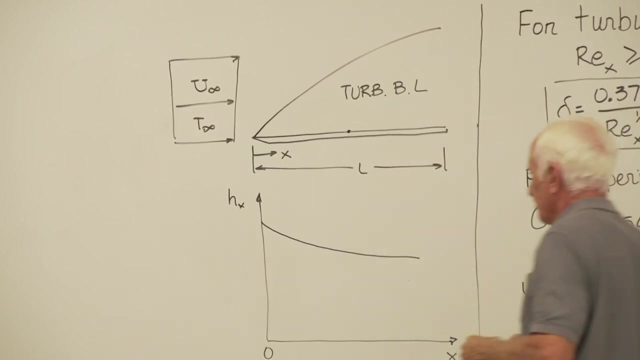 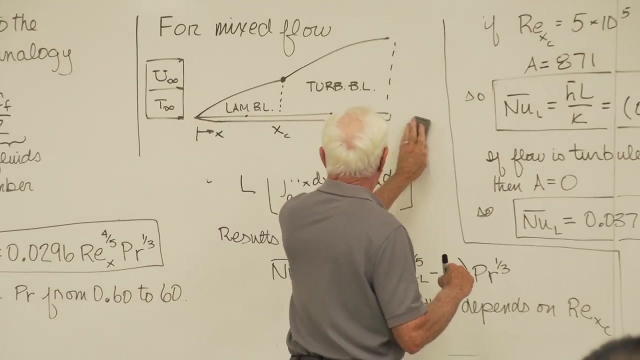 It goes down like that For turbulent flow. it looks like this: It doesn't quite go down as steep, It's flatter. It's flatter Laminar flow 3. So H X drops off more dramatically. 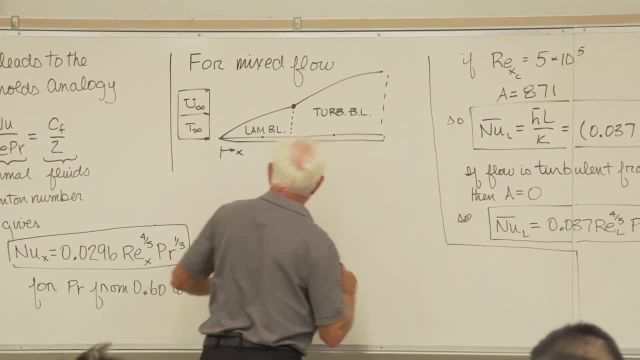 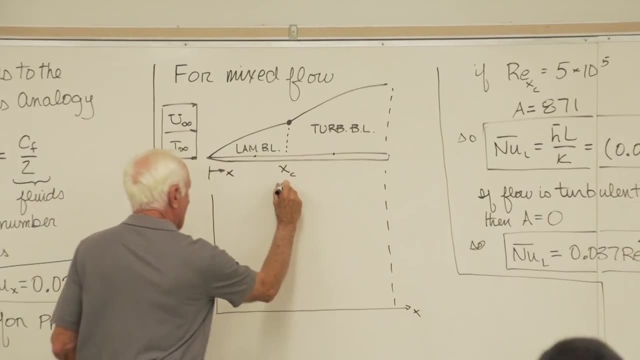 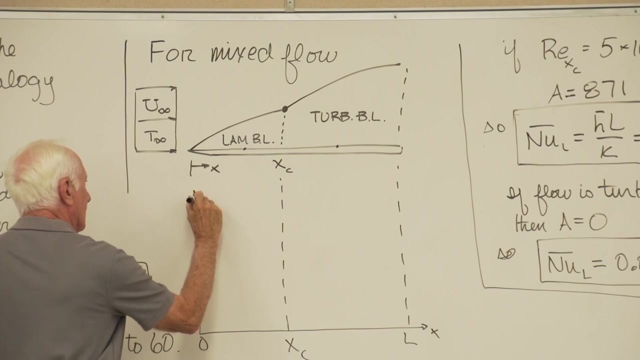 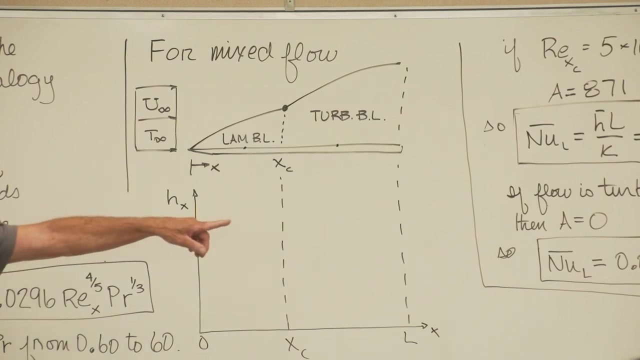 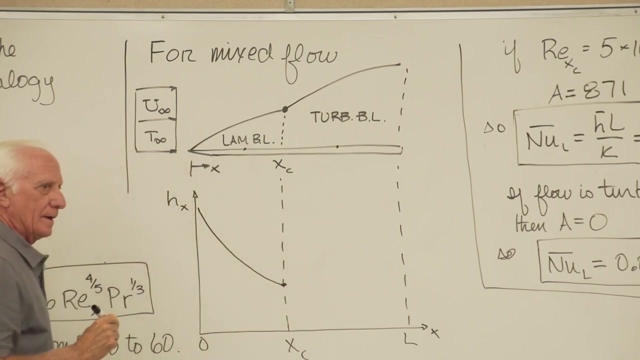 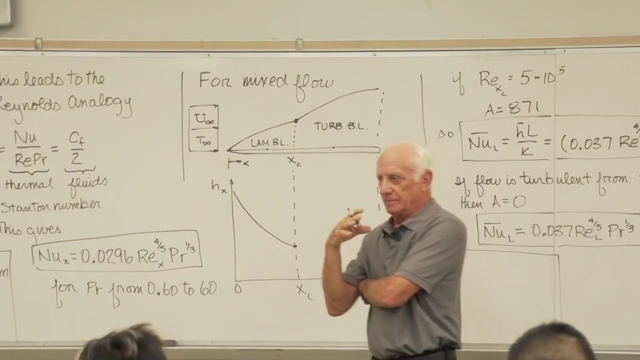 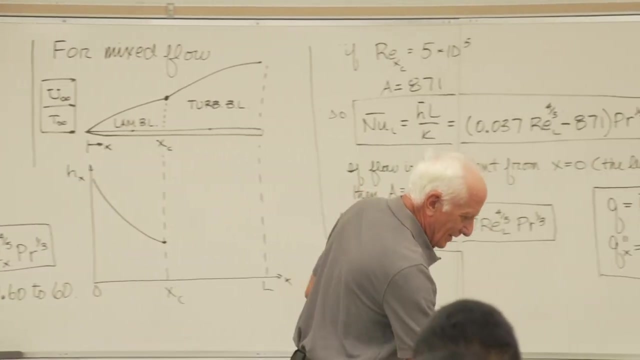 Mex flow laminar boundary layer picture over there. At that point the flow transits to turbulent. Dramatic things happen. Turbulent flow: there's a lot of vertical mixing in the fluid, The vertical flow. laminar means lamina. 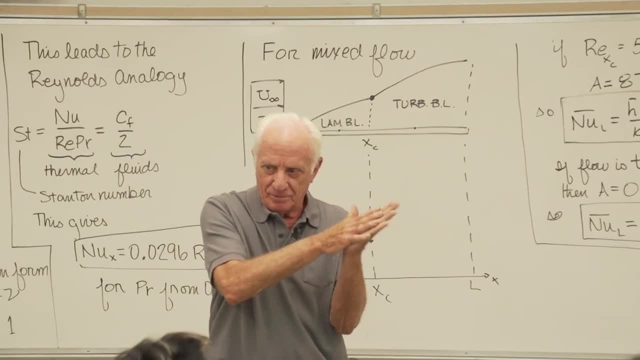 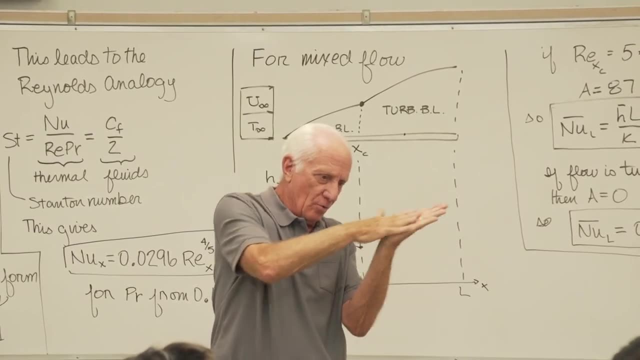 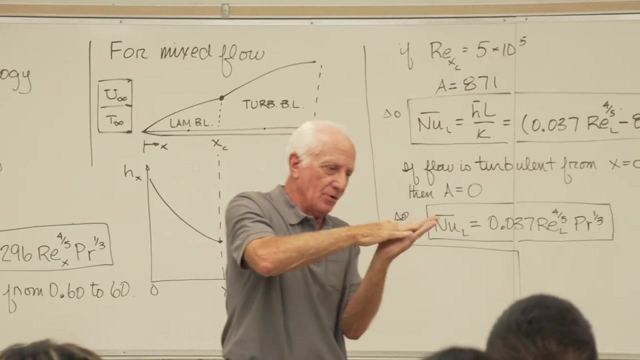 Lamina means like paper in your notebook. They slide over one another very easily. The molecules of the fluid slide over one another very easily: Turbulent flow. there's a vertical component of that velocity, so now it's rougher. There's more vertical mixing. 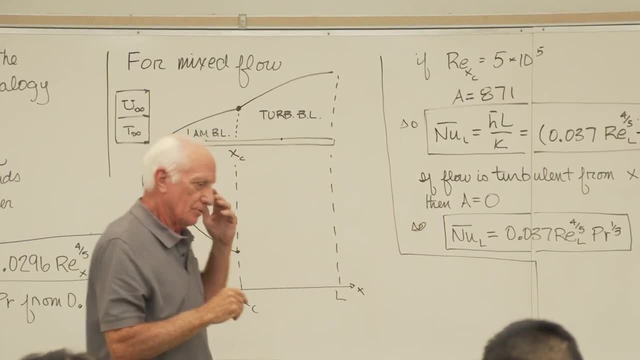 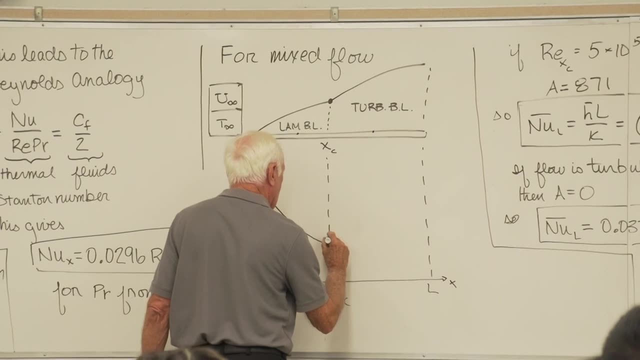 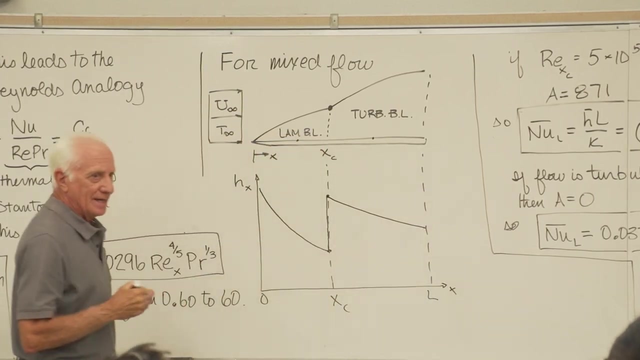 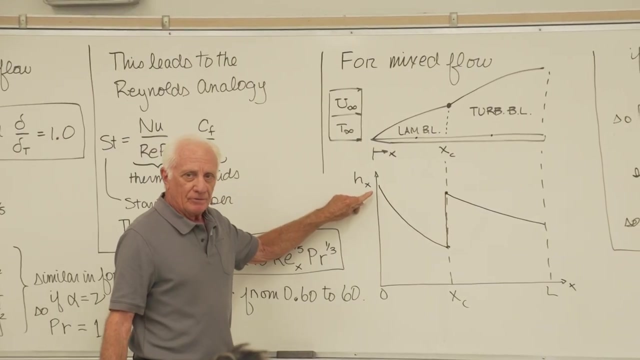 That creates better heat transfer. So now, when you get to turbulent flow, bam h sub x goes up dramatically. Now it follows that. So that's what happens in a mex flow plate situation. Hx really good near the front of the plate. 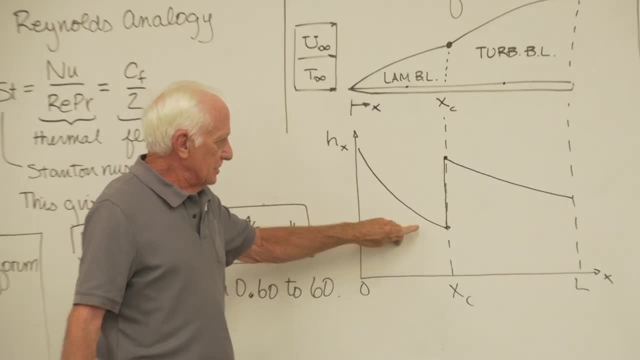 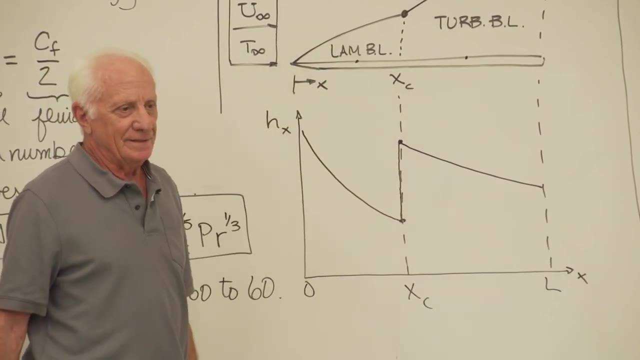 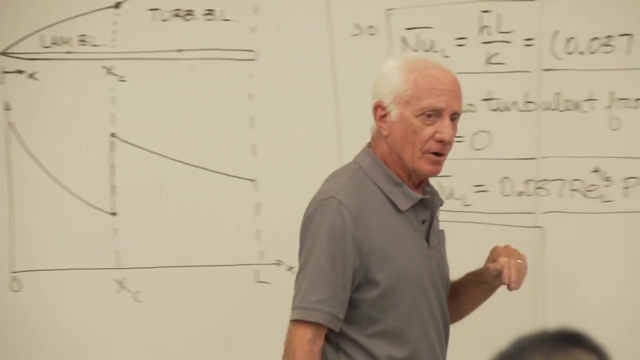 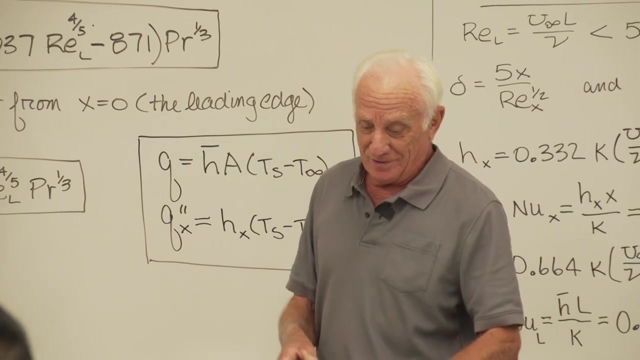 really good. the best Hx goes down until it reaches X value. Now the flow transits to turbulent Bam. The heat transfer goes up again, But now it declines at a more gradual rate in the turbulent part of the boundary layer. So that is why, again, 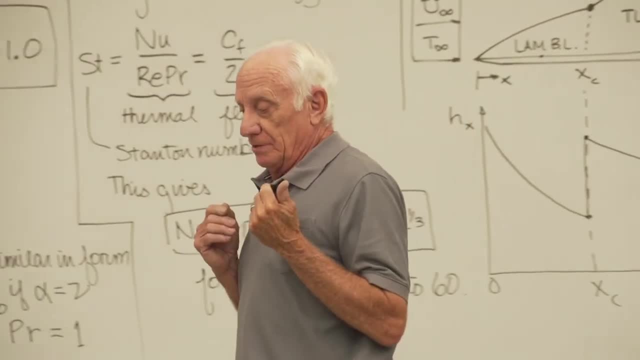 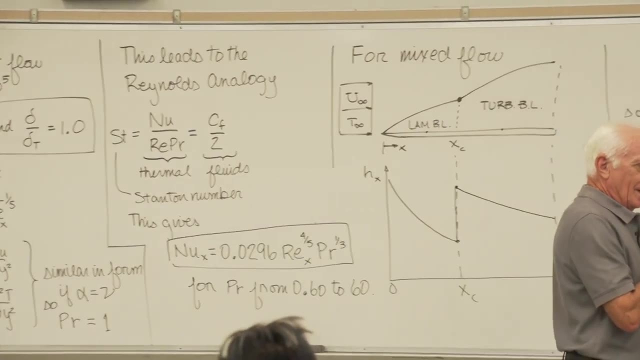 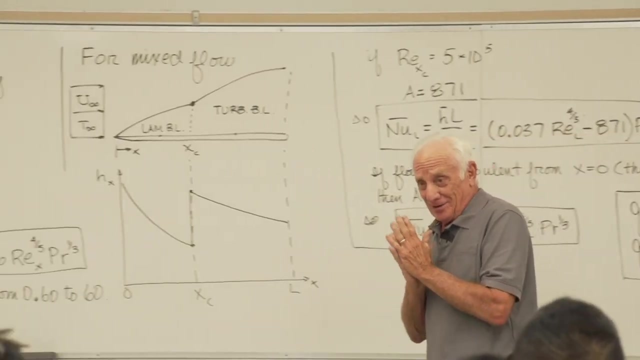 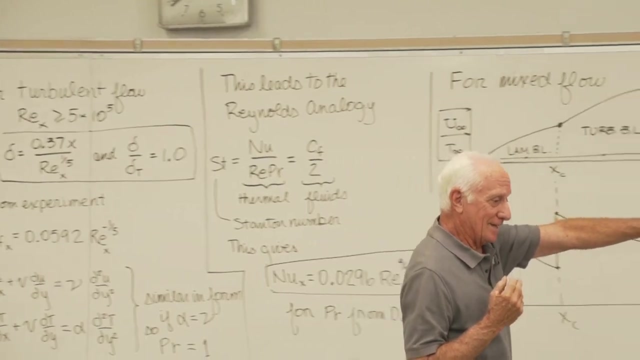 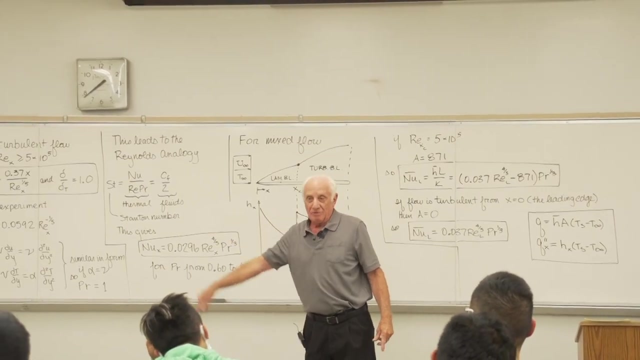 if you want good heat transfer, you want turbulent flow. If you want good heat transfer, you want turbulent flow. If you want to reduce the drag on a body, then you want laminar flow. So fluid mechanics reduce the drag. I want laminar flow. Heat transfer: I want good heat transfer. I want. 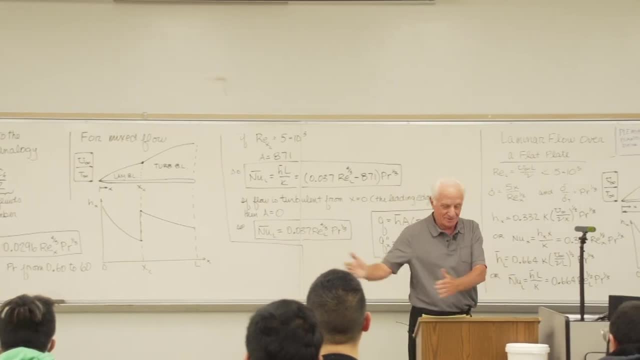 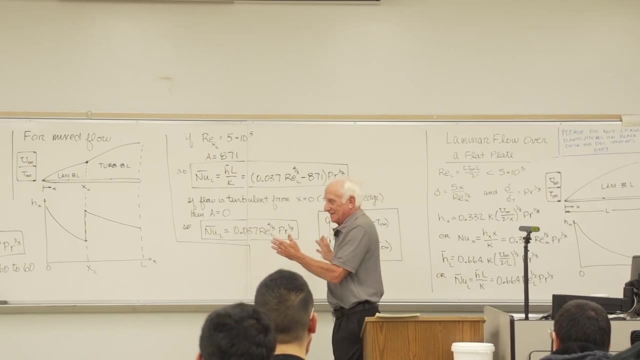 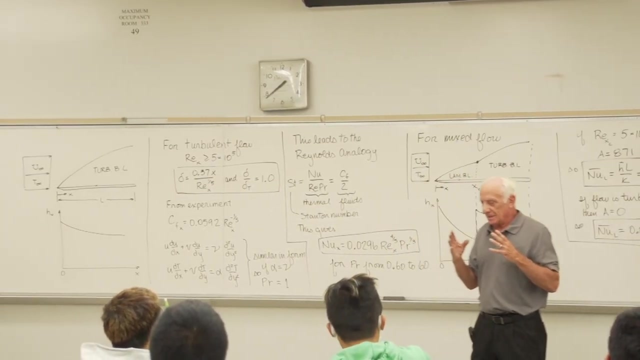 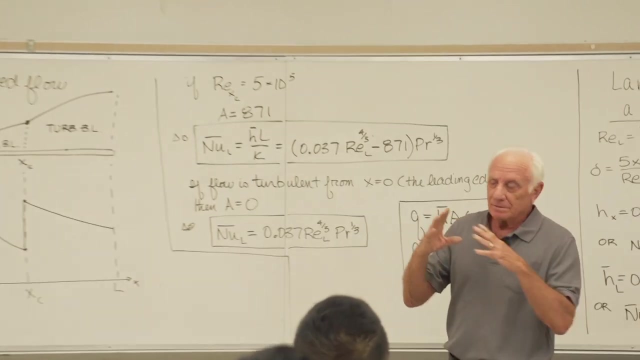 turbulent flow. Just the opposite: Fluid versus the heat transfer. Okay So, this is the first part of Chapter 7, flow over external surfaces. Our next topic is going to be flow over cylinders, So it'll be flow not over flat plates like pipes, Cylinders. Okay So. 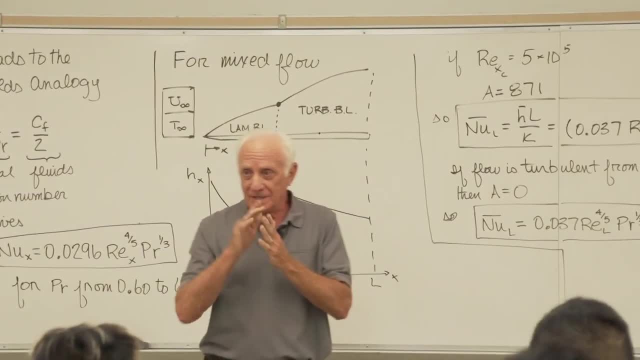 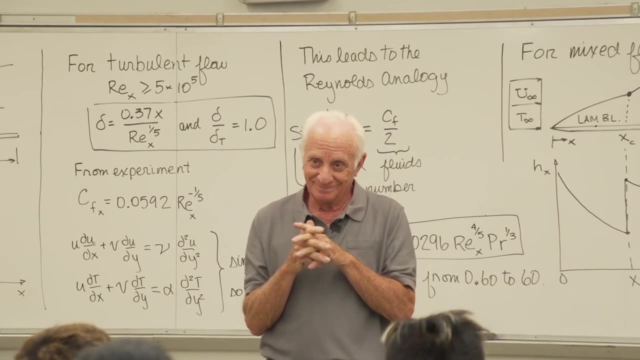 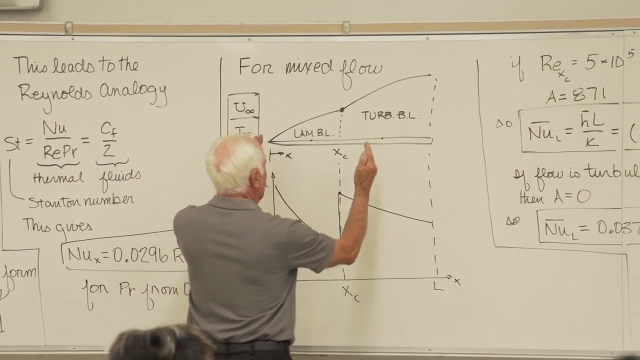 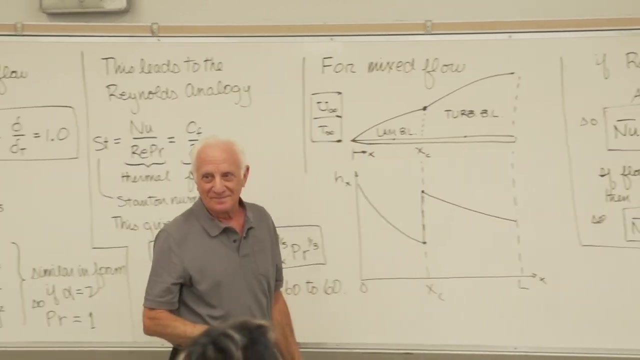 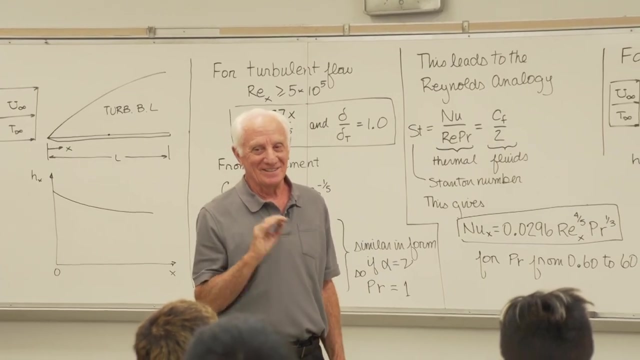 we'll do that next time. We're going to stop right now. One question: Yeah, What? Oh, yeah, Yeah, You would put this distance in this equation right here. Is that what you're thinking about Now? tell me why you're concerned. I think I know why. Tell me why you're concerned.